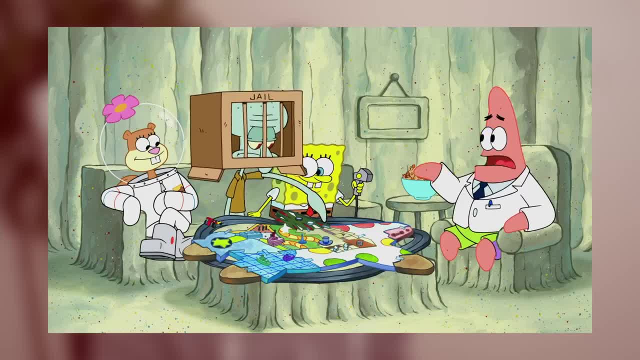 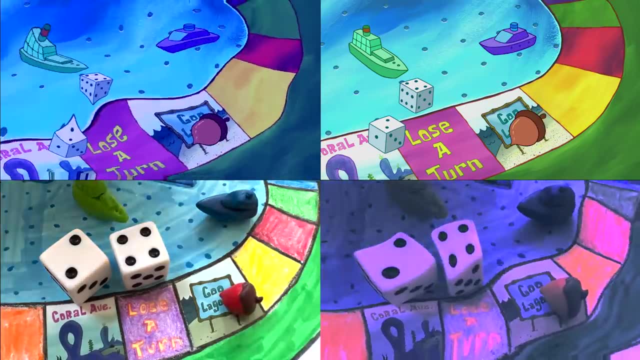 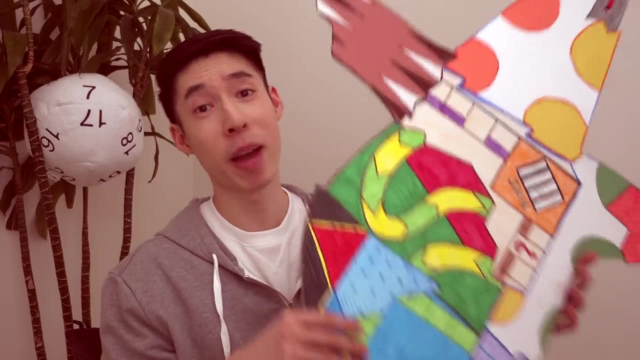 Recall this Spongebob episode when Patrick makes a board game and then invites everyone over to play. Well, I made that game in real life. The game is called Patrick, the Game Might. I suggest garbage, And today I'm going to show you exactly how I got this game to match the one from the show. 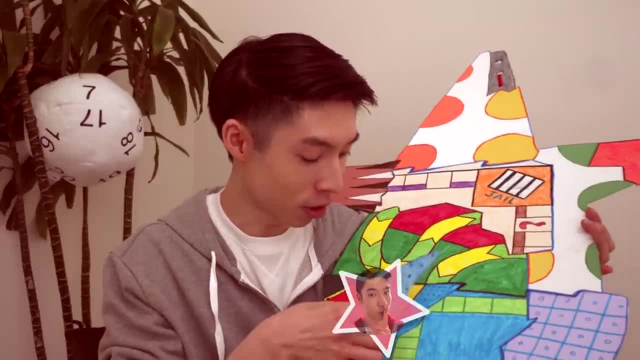 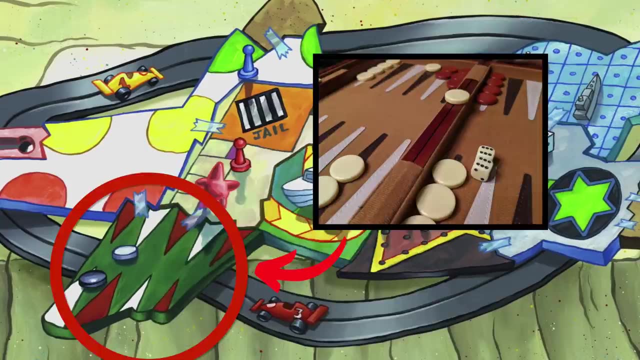 Wow. And then I'll reveal some hidden features and show you how my friends react when we try to play this game. At first glance, the board looks like a combination of Battleship, Backgammon, Monopoly, Chinese Checkers and Twister. 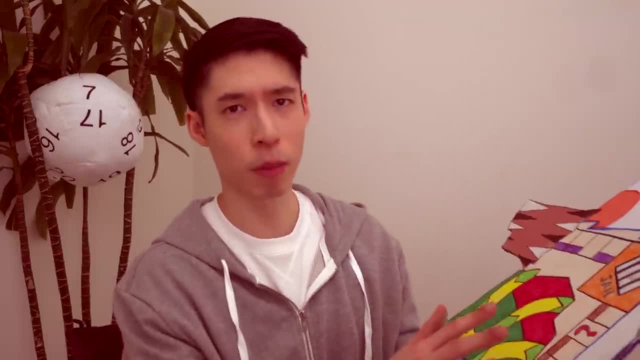 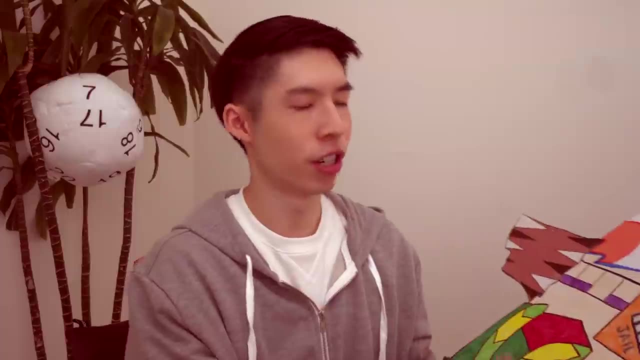 But you know what? It's actually not that straightforward. There are a lot of things that were physically challenging, to make, Almost impossible, But I made it work, And today I'm going to show you exactly how I did that. Sure, some of the parts were a little impromptu, but I tried my best. 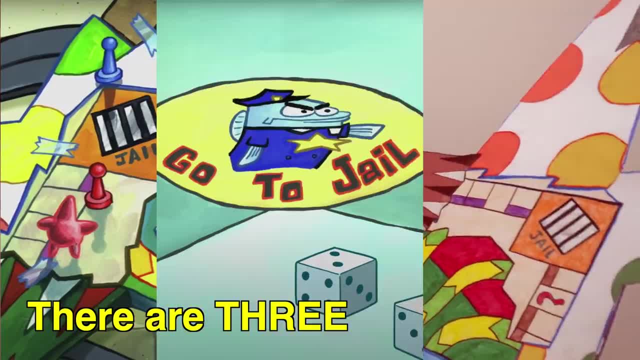 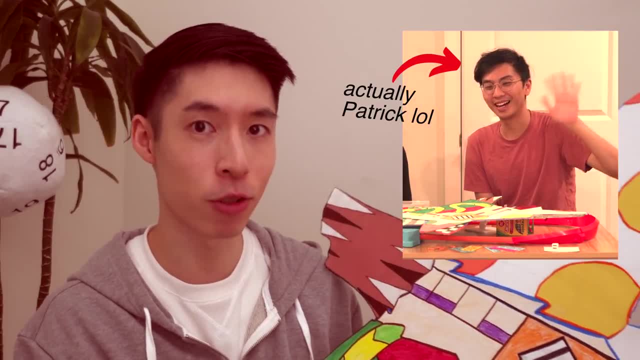 And I'm going to show you how I reconciled a lot of inconsistencies on the board. Afterwards, I'm going to show you how I organized the rules to match the rules from the episode and then reveal it to my friends, one of whom is actually named Patrick. 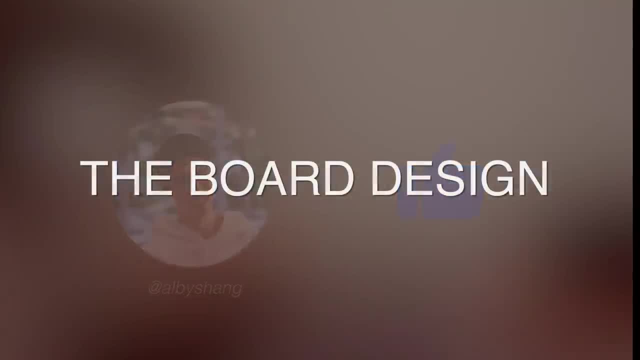 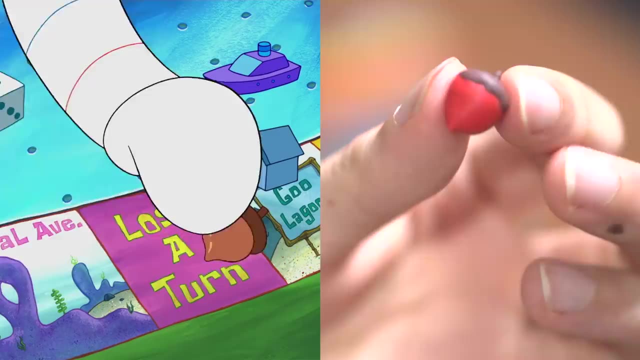 My name's Alby and I like to make board games. Now let's get started with the game design. The feeling I get from this board is that it's supposed to be a makeshift combination of random games and rules chaotically stitched together. 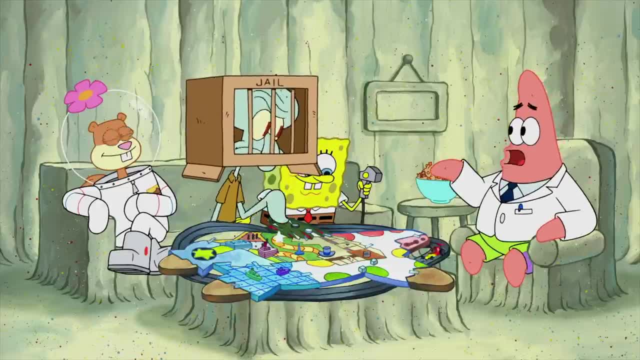 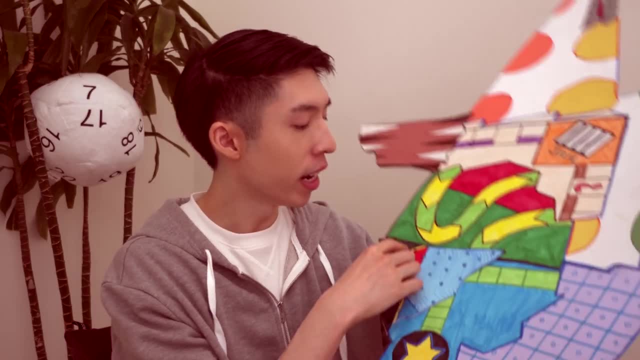 to form this Patrick, the Star-shaped board with a race car track underneath. But if you look closely, you would realize that Patrick would have had to measure each of the boards thickness and make them match, as well as cut them out in perfect zigzag shapes that would seamlessly fit together. 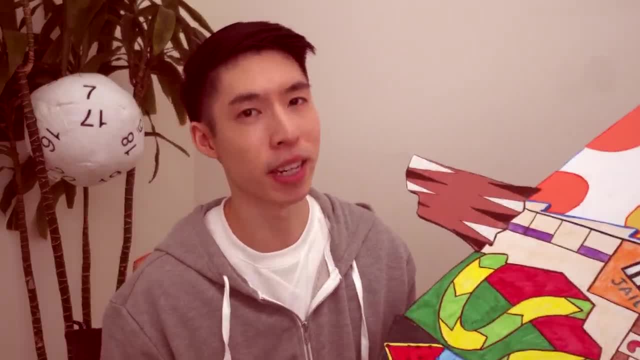 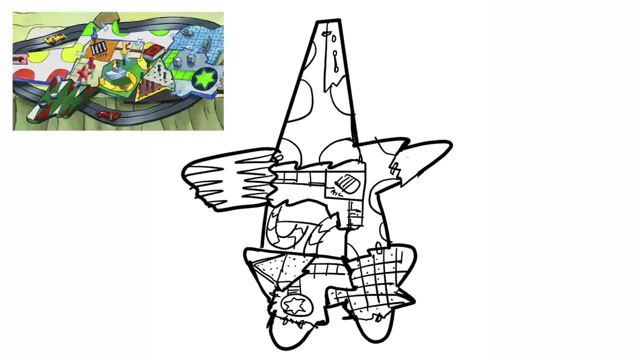 That is really hard. Luckily I'm not copying how I think he made the game, just how it looks. The first step of making this game was deciding the size. The main component that has a fixed size is the race car track. I looked all over Amazon and eBay trying to find a race car track that was one loop across. 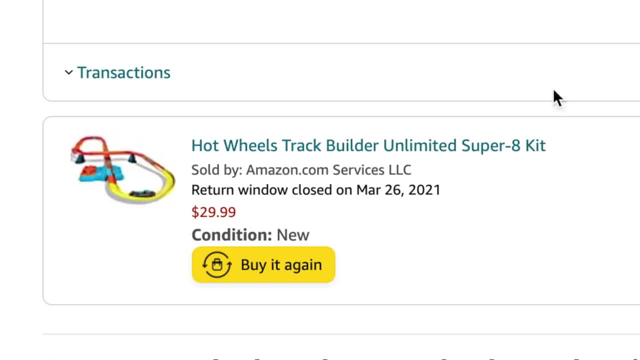 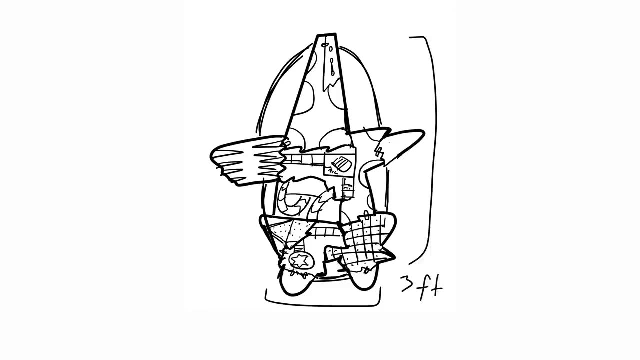 and even a black one, but I finally gave up on the color. Eventually I found one on Walmart that was selling for about $30 something, so I immediately bought it. Once it came in the mail I put it together and measured it to be about 3 feet long and 1 foot. 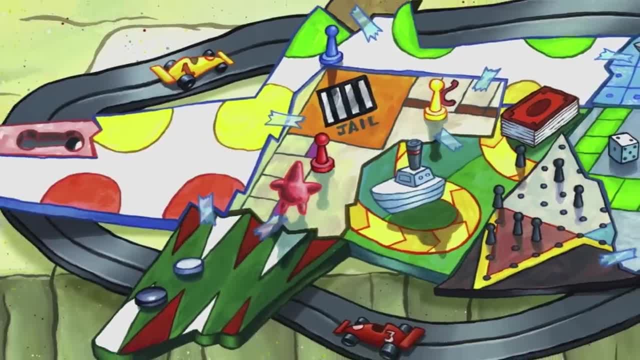 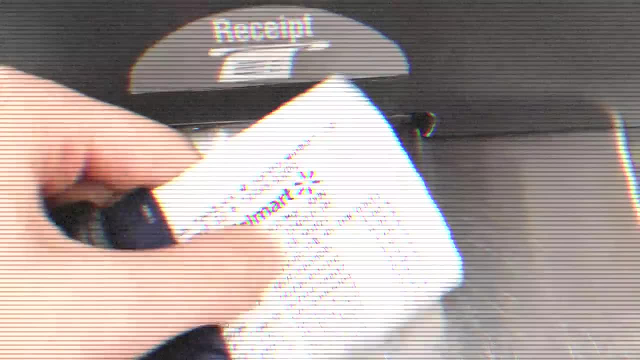 wide, which meant that my board had to be longer than 3 feet and wider than 1 foot, with the arms extending out and the head popping out. So I went arts and craft shopping and then went straight to work. To make it easier, I just made the arms the same width as the foam board that I got. 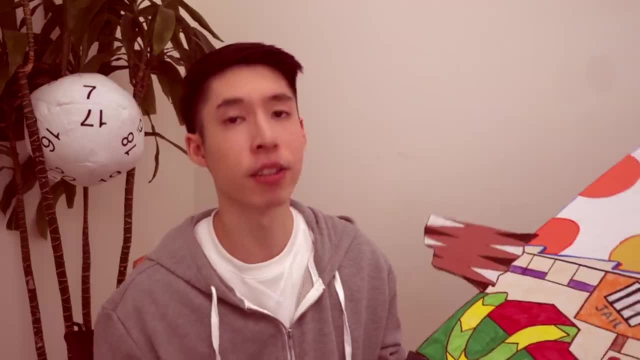 and then I attached some additional pieces of foam for the head and the feet. I used a mix of construction paper, crayons, colored pencils and markers to draw out the entire board. But here's where things get tricky. You see this jail cell. 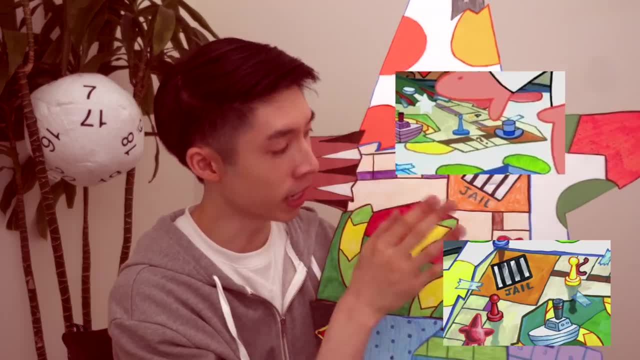 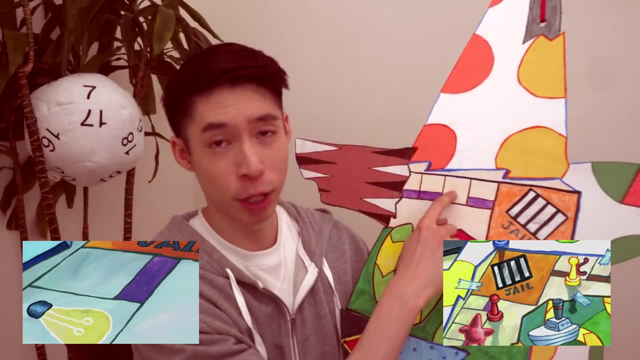 When Squidward landed on this space and then it zoomed in in the cartoon, the space looked like this: How do I reconcile that? Not only that, a light bulb appeared on the spot, and then this question mark chance turned into snacks. 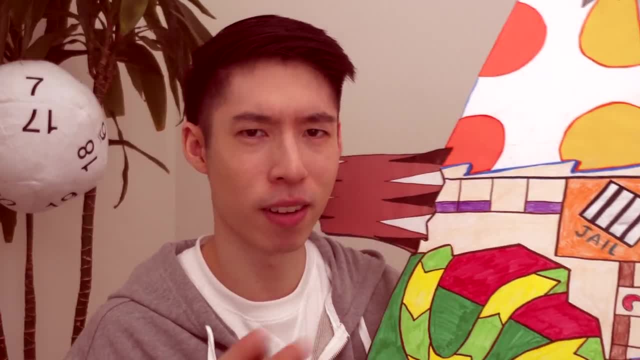 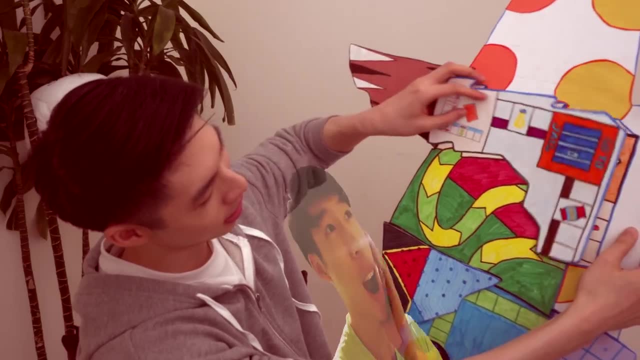 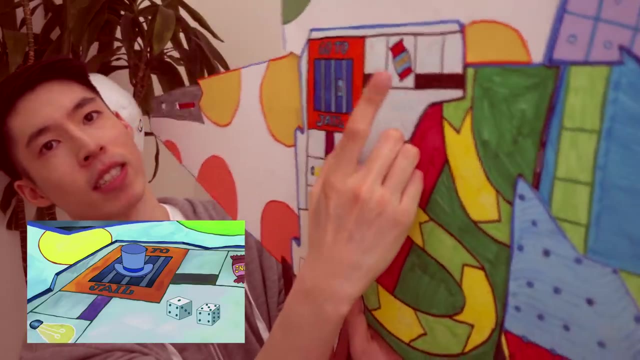 In a cartoon, that's fine. but for real life, How do I make that work? The way I did it is by creating an overlay layer. This piece- Ha ha, Go to jail- matches the cartoon. And now there's snacks and the light bulb. 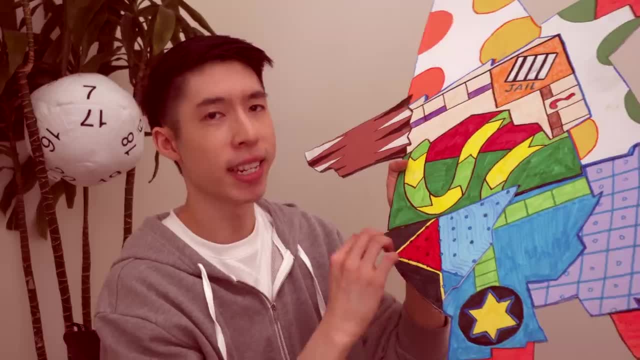 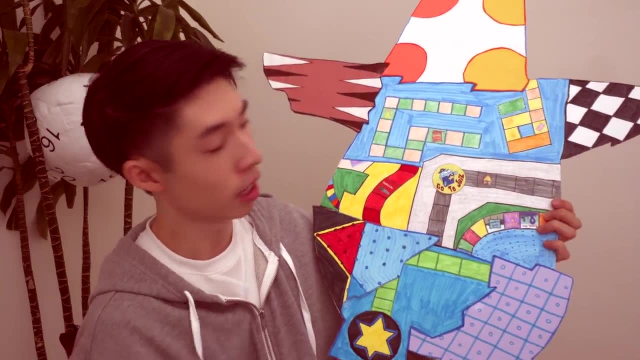 And that's basically what I did for a lot of inconsistencies. I had to cut out exact shapes of the board and then tape it on, And if you look closely, this is already an overlay layer. If you take it off, you'll see a lot of parts of the board. 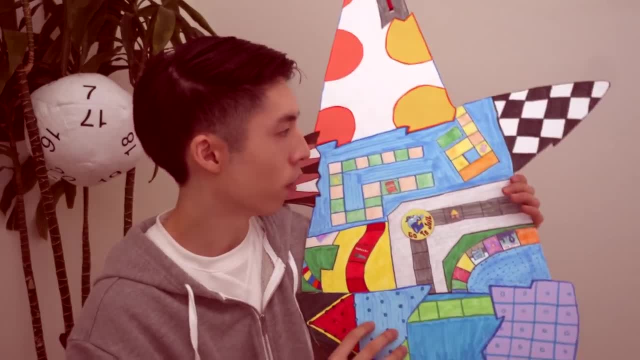 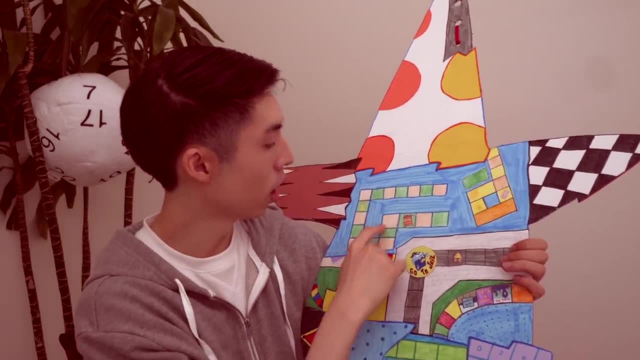 that weren't on the original but were shown in the cartoon. For example, this spot is Spongebob's driver's license area where he loops around, And there's this green spot where Patrick lands on snacks And this part where Patrick lands on snacks. 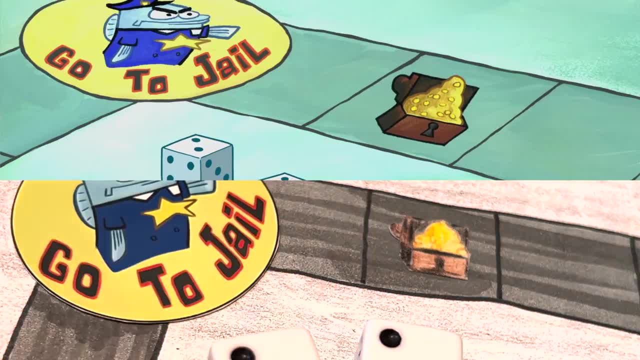 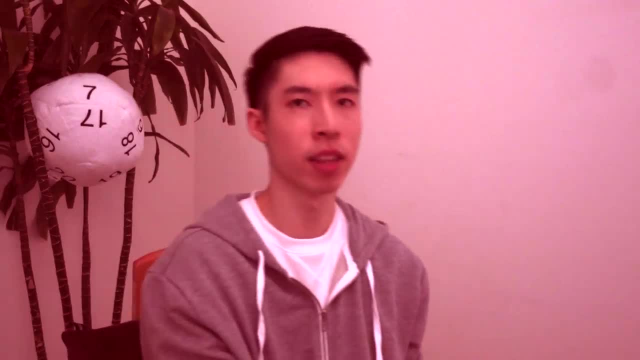 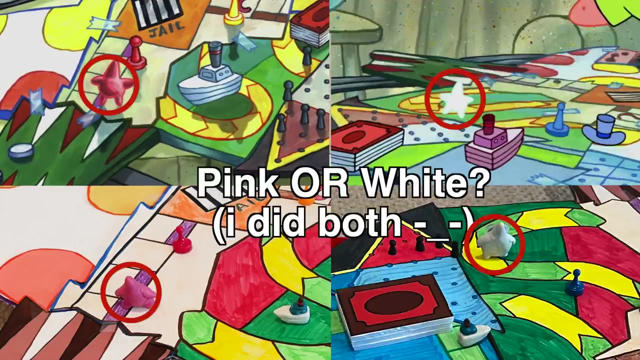 And then she does surgery here. Of course you can't make everything in the right dimensions and proportions because in the cartoon pieces just get moved around all the time And their dimensions just change randomly. Like Spongebob's little boat piece. In some angles it just seems like it makes perfect sense to make it that size. 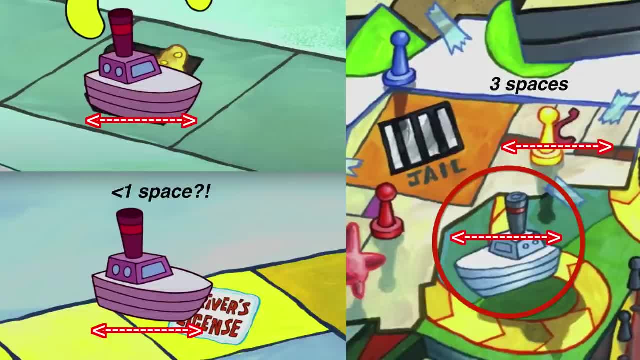 And then when you zoom in in the cartoon, there's suddenly a different size. And I have to admit there were other parts of the board that I just couldn't address, Like when the snacks popped out of the box. I couldn't get them out of the box. 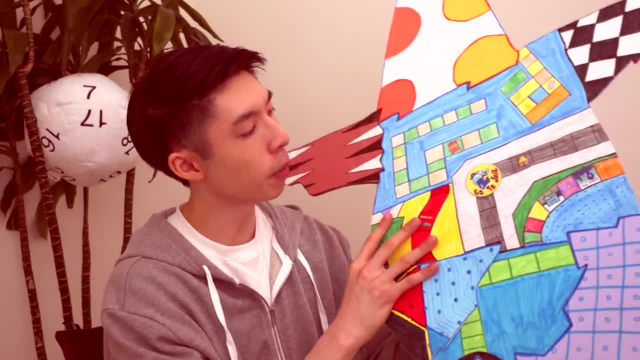 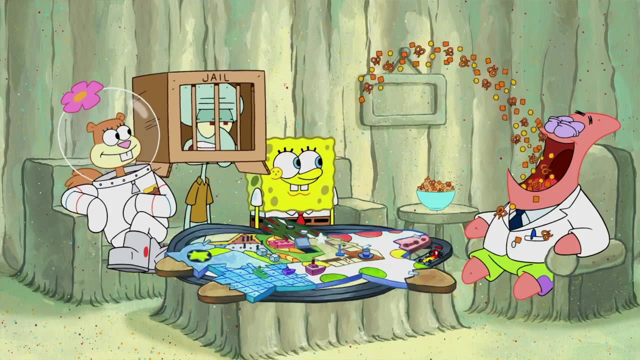 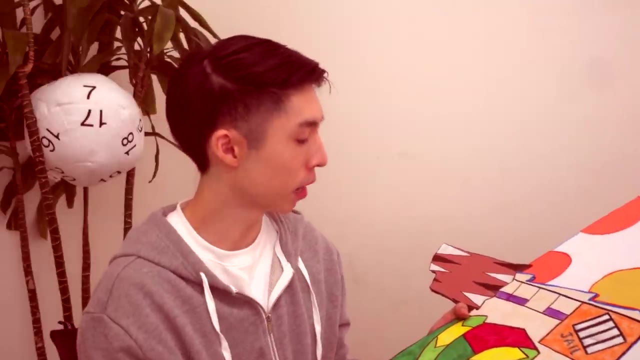 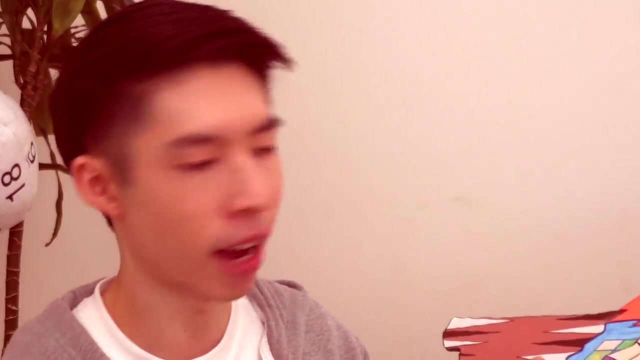 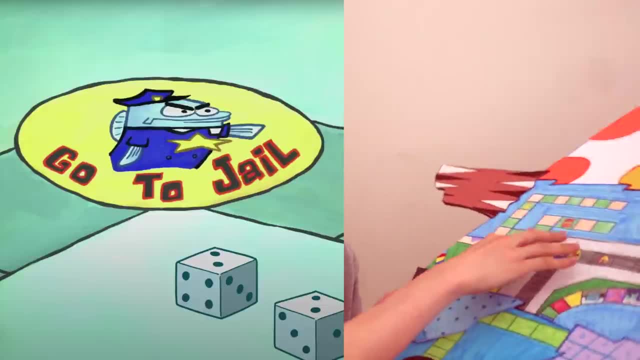 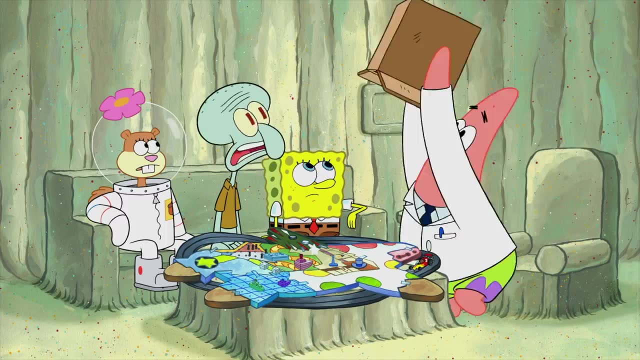 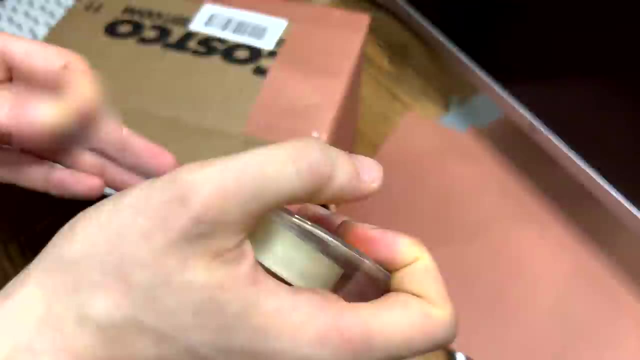 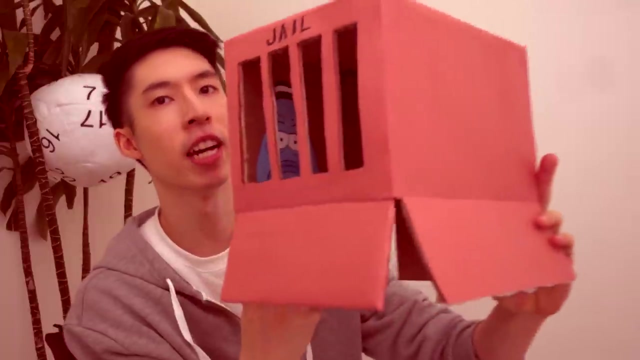 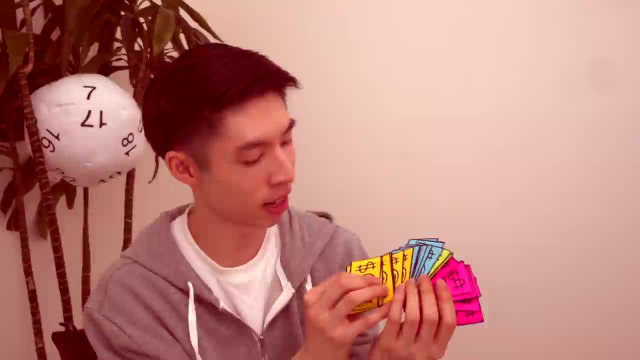 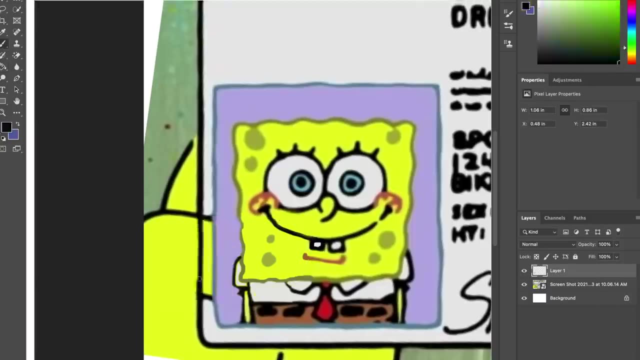 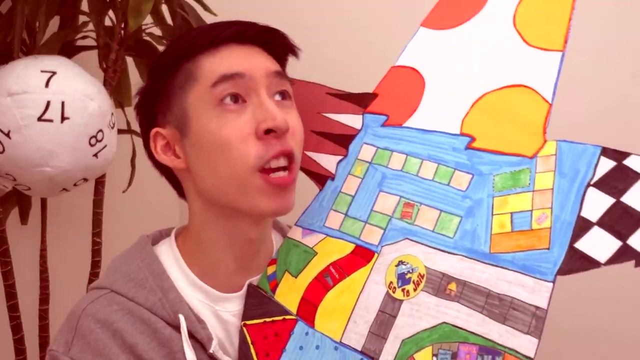 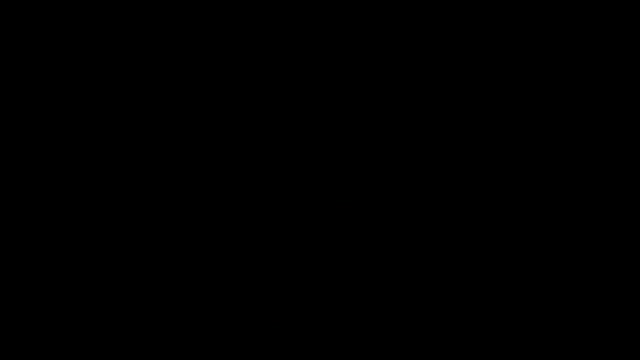 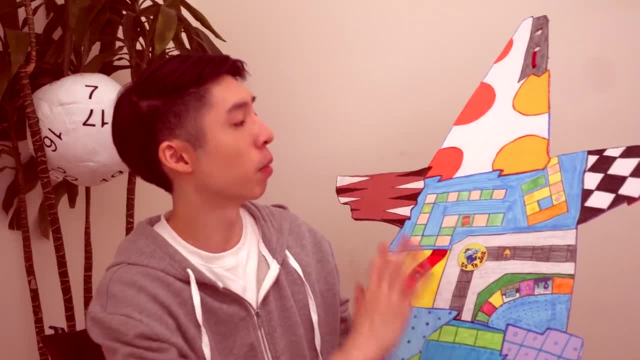 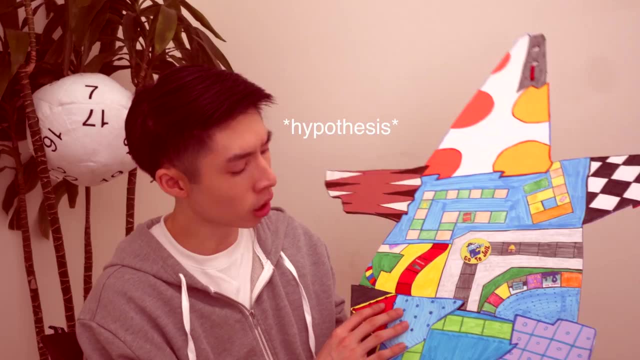 them out of the box, Even though the game is a bunch of different games stitched together. a lot of these games are never touched, like Battleship Batgaming, but some are like Operation. I'm thinking they would come into play other characters like mr 분들이 or Plankton maybe. 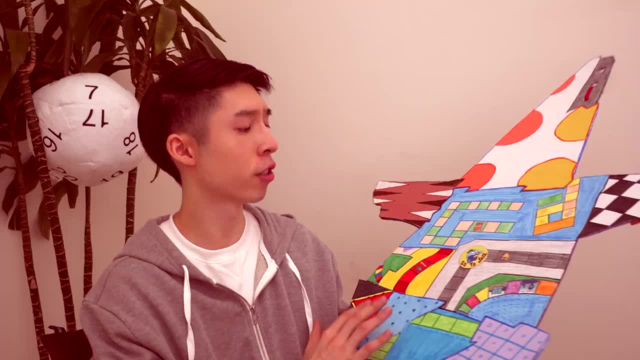 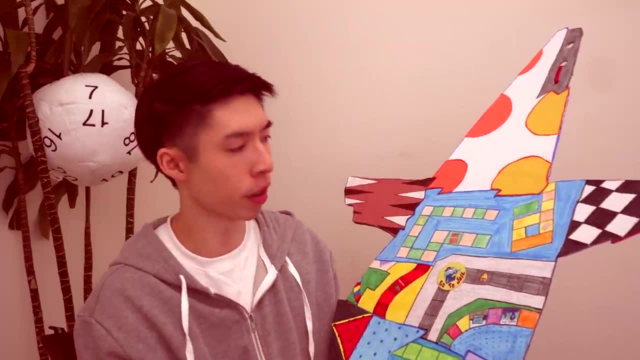 this battleship is for mr crab, who knows Either way. we see the player turns are be for the part. like Monopoly, You roll the dice and then you move the amount of spaces that you get. Once the dice, each player seems to have their own section of the board. they move on. 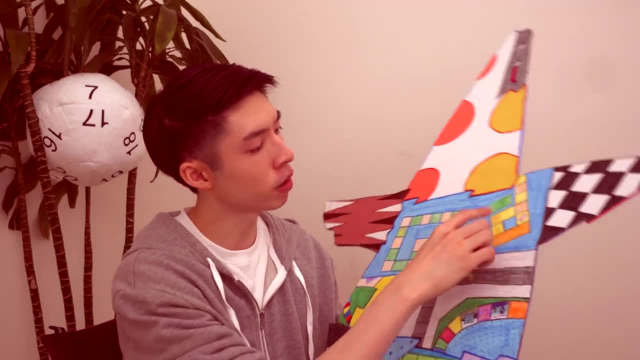 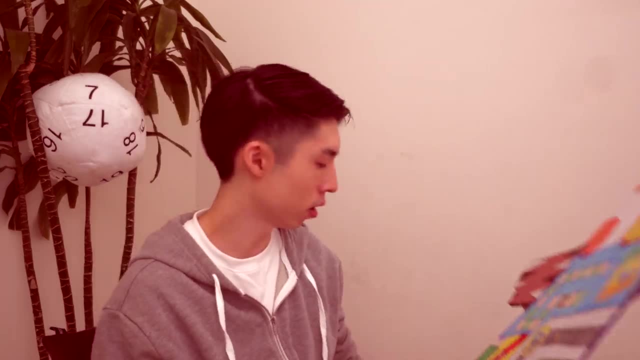 For example, Spongebob moves on this gray go-to-jail section and then moves on this yellow, orange, sponge-themed colored section. Hubert is constantly going to jail on a Monopoly-style board and Patrick is moving on also a Monopoly-style board and this green section. 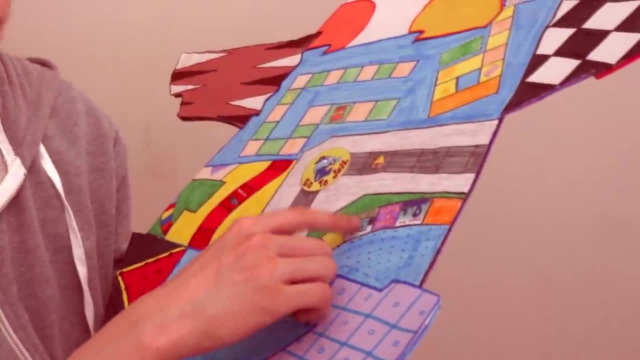 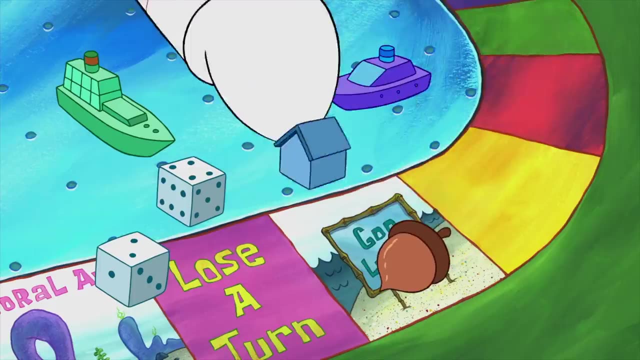 Sandy's play is the most similar to Monopoly, where she actually purchases property. I'll buy it. But for Goo Lagoon she gets a beachfront property without even actually having purchased Goo Lagoon in the first place. Beachfront property. 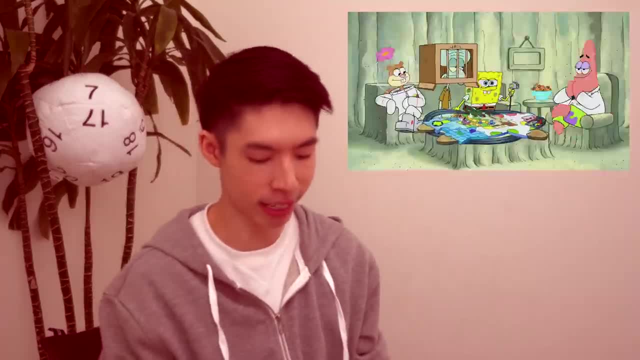 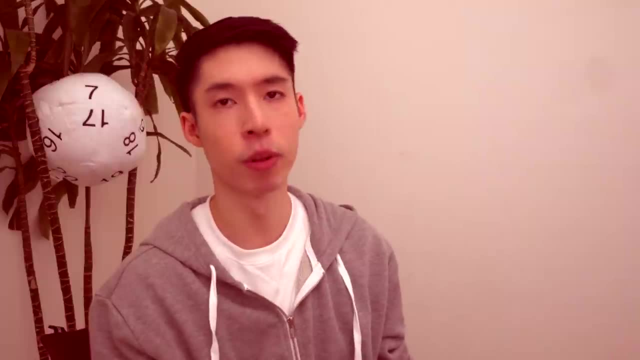 So it's not all like Monopoly. I did another watch through of the episode and I came up with some rules for the game. For the actual rules that they said in the game, I wrote them down verbatim bold. And for the other stuff. 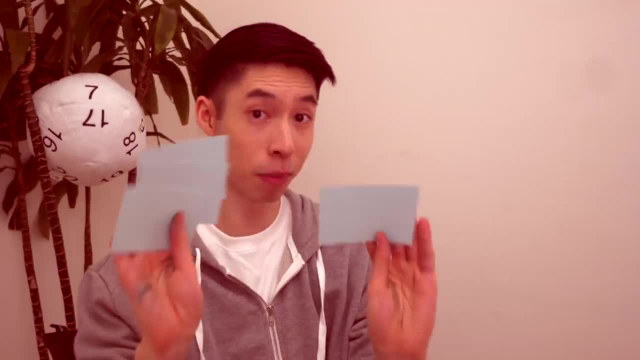 I just wrote down what I saw happen. All of this is on these blue cards, just like in the game. I even got some blank cards that you can use to write down your own rules, because Patrick is constantly crossing out and writing new rules. 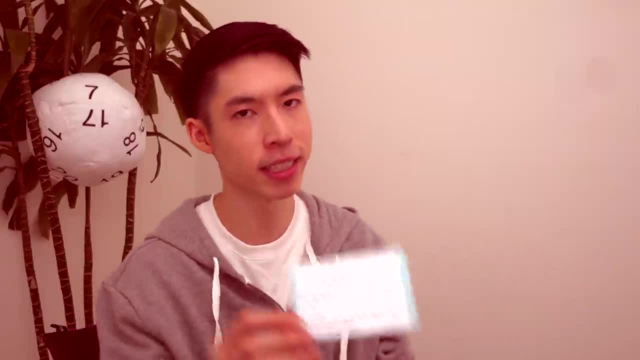 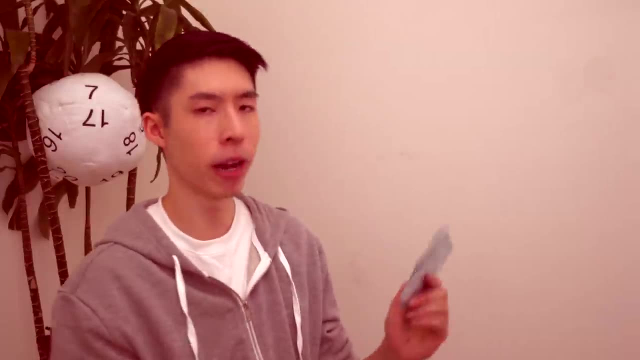 For example, when Squidward says automatic winner, Patrick crosses it out and then says no player may declare himself automatic winner. So I have that on here. But I also had to fill in some of the blanks because Patrick got interrupted when he was explaining. 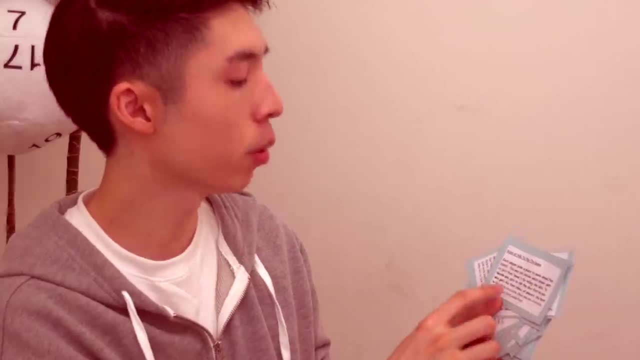 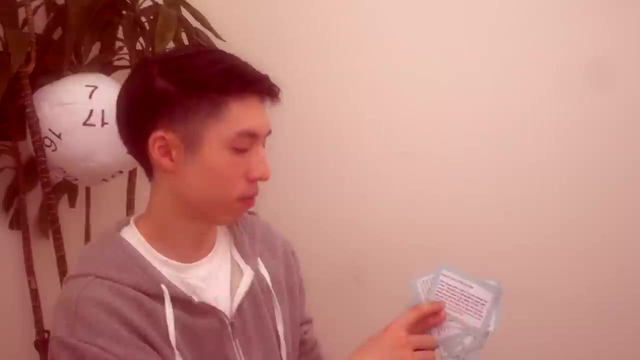 how to pick the first players in turn order. There's this part where he says to decide who gets to roll the dice first, to see who gets the first choice of players, and then he gets interrupted by Squidward. So I just said sitting in a circle. 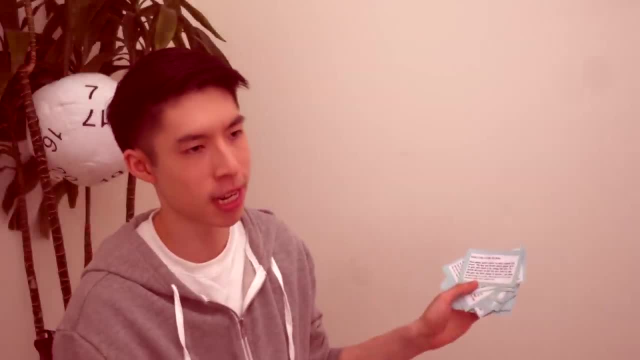 Once you're in a circle, whoever talks first picks first. I derived that just because there was that part where Squidward was in jail and they had to say his name in order to get him out of jail, So I thought that was similar enough. 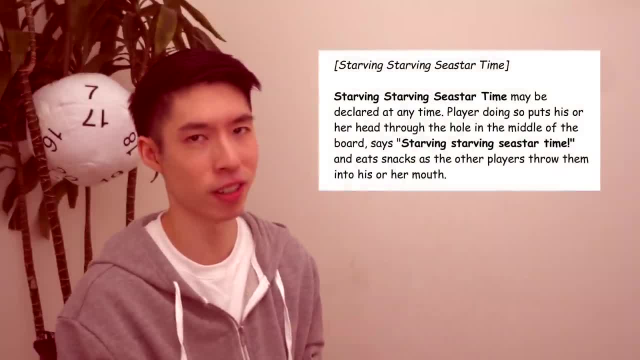 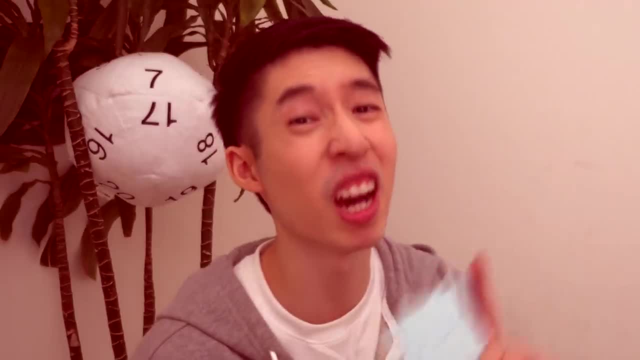 And other parts. I just wrote down what I saw them do. For example, there was that starving, starving, see star time, where players just threw snacks into Patrick's mouth. Starving, starving, see star time. Speaking of which, 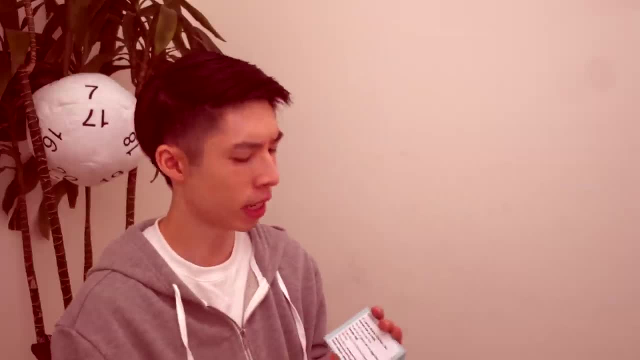 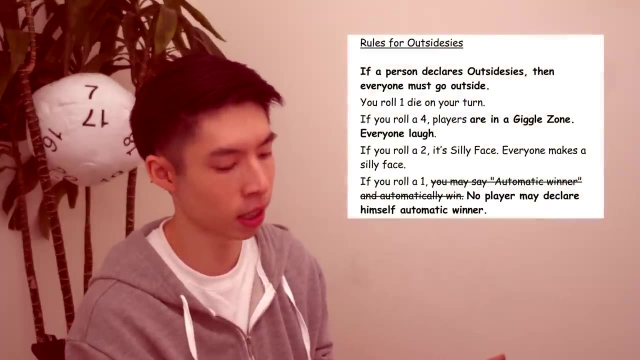 I also had to carve open a hole in the middle, And an interesting part of the game is outside-sies. Okay, I'm going outside. Outside-sies follows a whole new set of rules where everyone has to go outside once it's been declared. 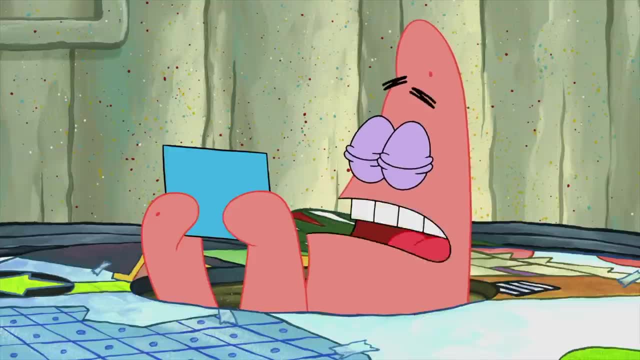 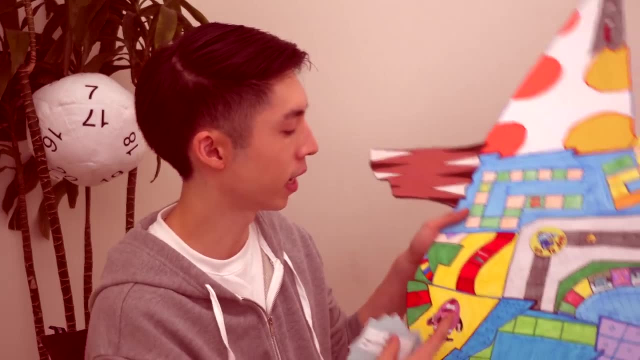 If a person declares outside-sies, everyone must go outside. You no longer roll two dice, You roll one, And for each roll, everyone has to do basically the same thing. Lastly, there was a part of the game where Sandy lands on this do a surgery spot. 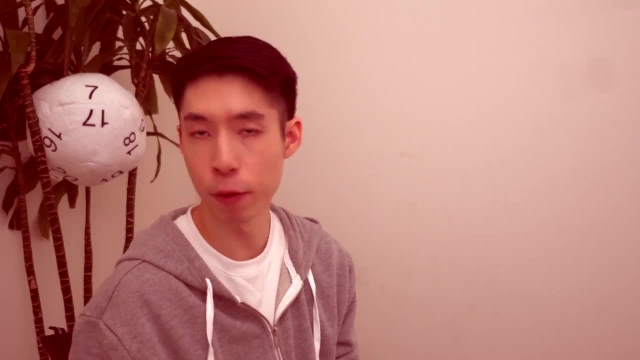 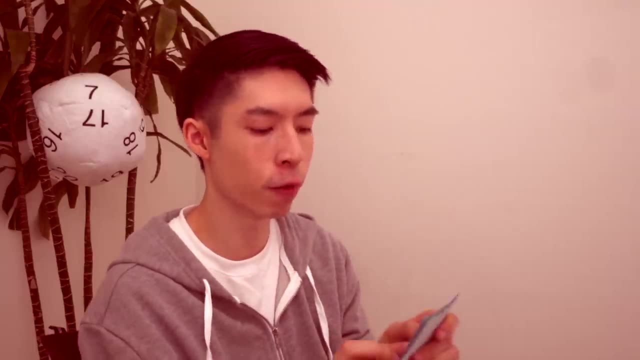 Patrick says that she has to choose from one of four surgery cards, then perform that surgery. She lays Squidward on the table and then does an operation. on this operation- fish. The surgery card said: remove thin bone from player to your left. 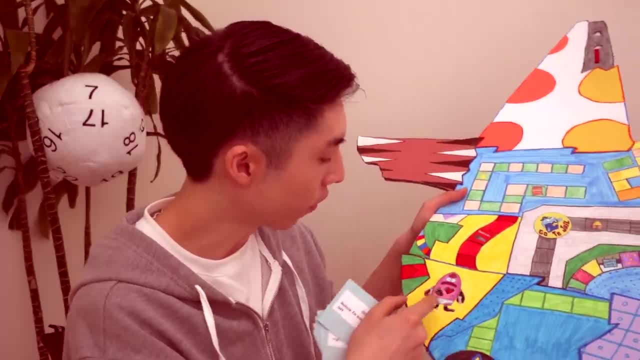 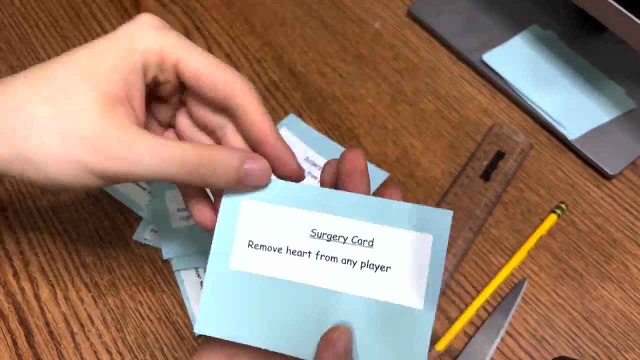 So I made that. But there were only four surgery cards in Patrick's hand and there are seven different spaces here: One, two, three, four, five, six, seven. So I took the liberty of making more surgery cards so that all of them could be picked. 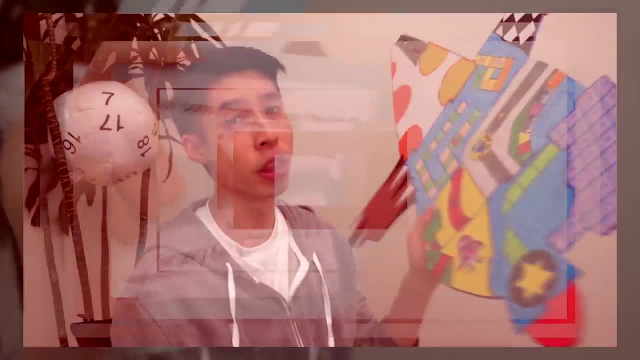 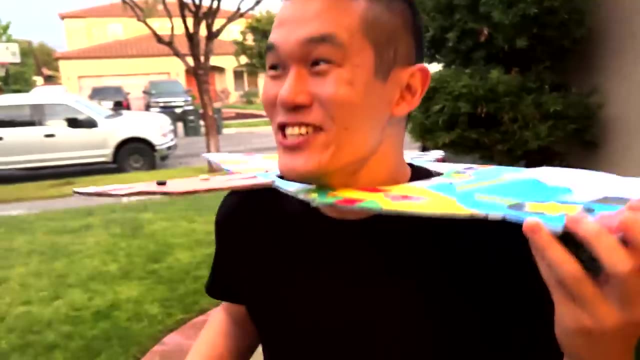 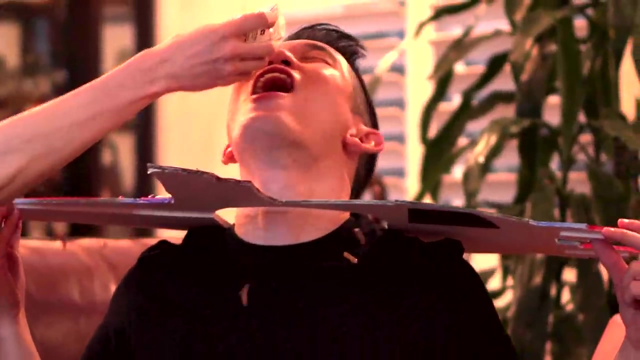 And I followed the similar format of the original surgery card. With the board finally done and the rules typed out, it was time to reveal the game to my friends. This is Sean, my silly cousin, And, as you might guess, he's a 10 out of 10 SpongeBob enthusiast. 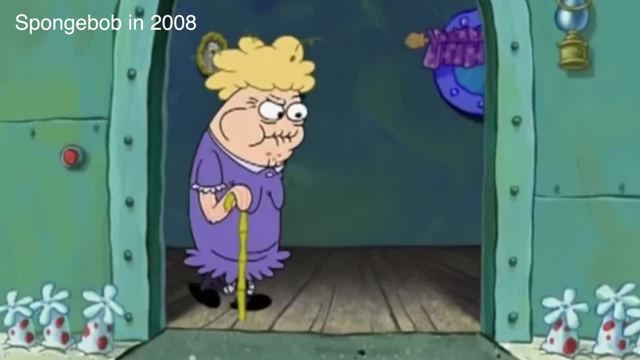 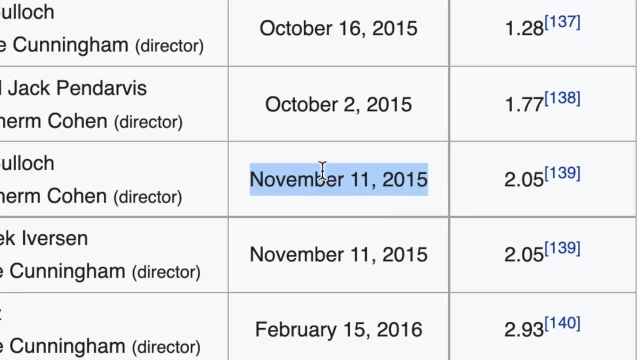 but mainly the vintage stuff from the 2000s. When I first revealed the game to him, he was actually slightly confused because he hadn't seen this episode before, which aired in 2015,. I later realized, And if you didn't know, 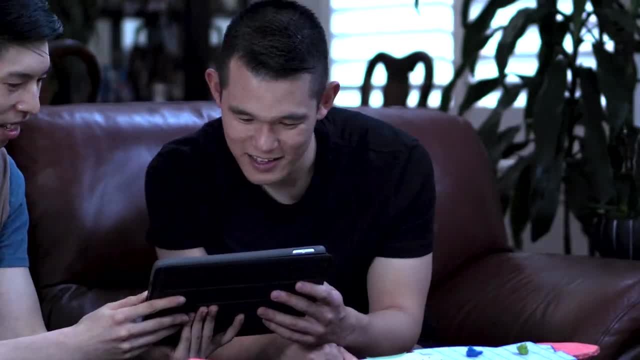 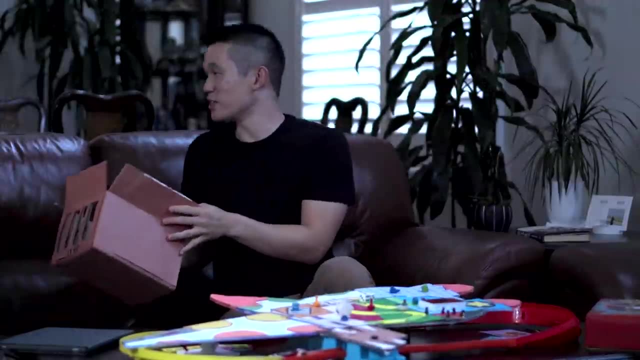 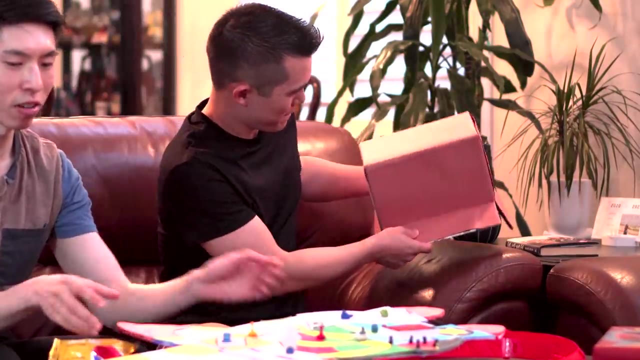 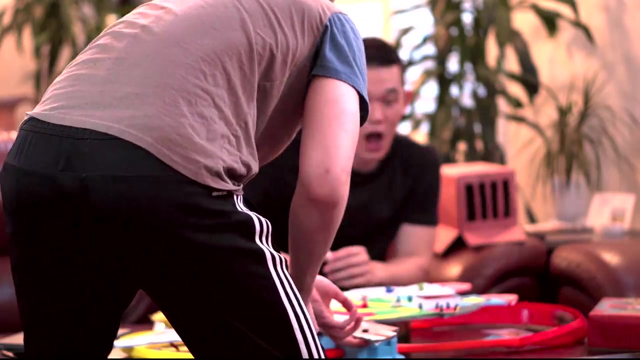 new SpongeBob episodes are still coming out these days, So I played it for him on my iPad before getting his feedback. Okay, so we're looking for accuracy. How close is this game to the one that you just watched? Okay, Whoa. 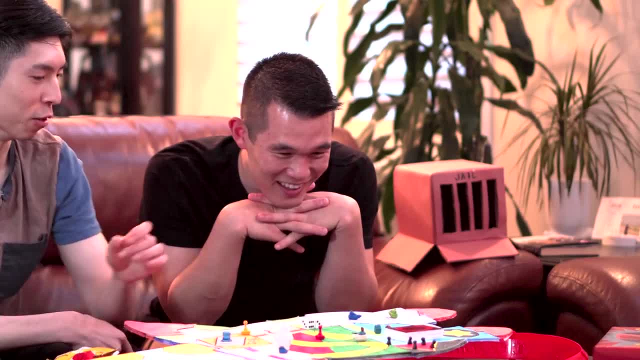 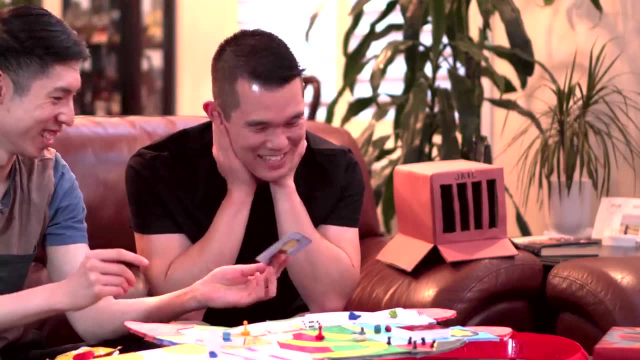 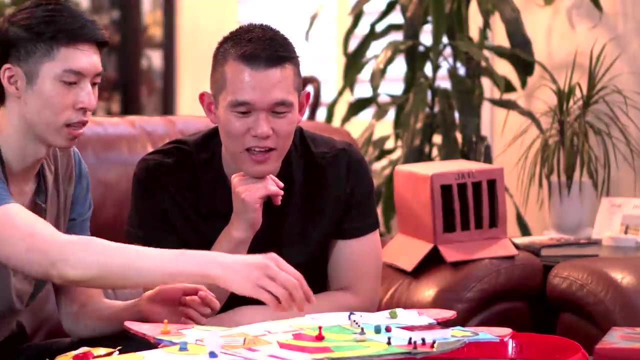 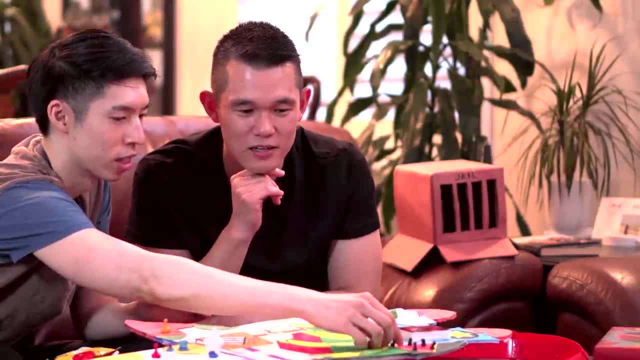 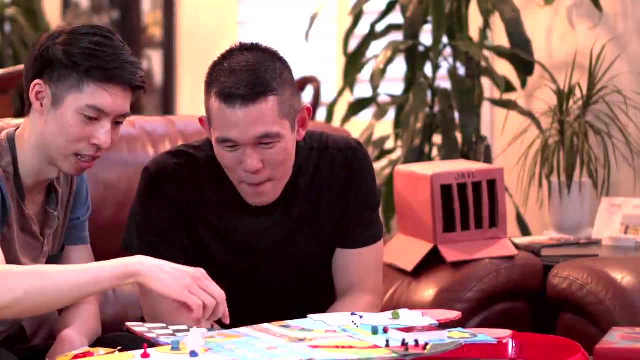 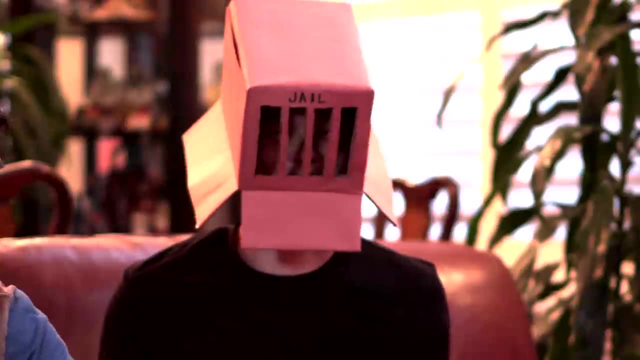 Because on the board it has many different versions In order to capture all of that. This is the part where SpongeBob goes and lands on driver's license And this is Sandy who's the acorn. I couldn't fit. I'm in jail. 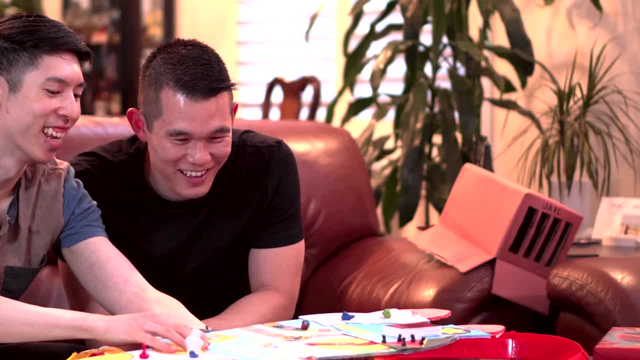 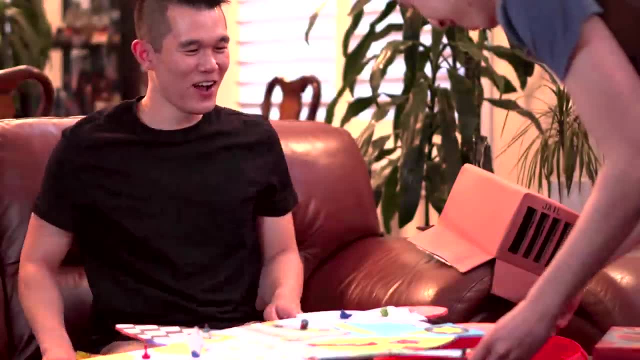 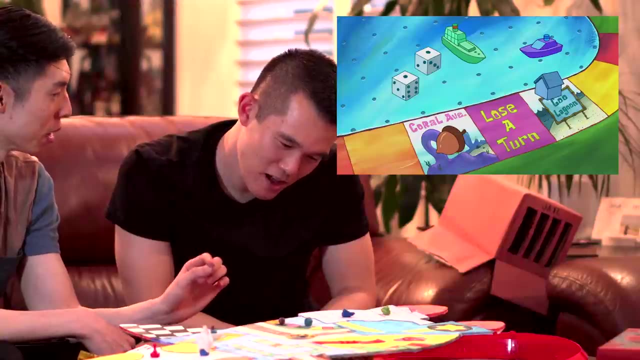 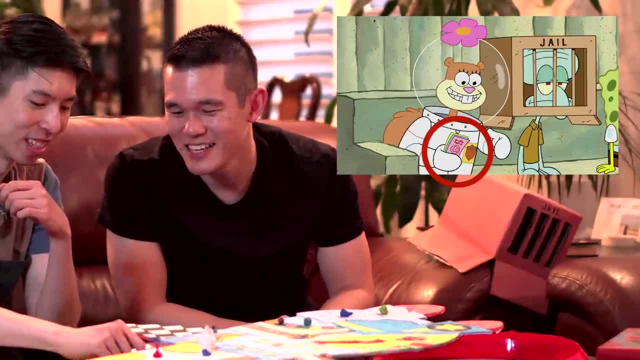 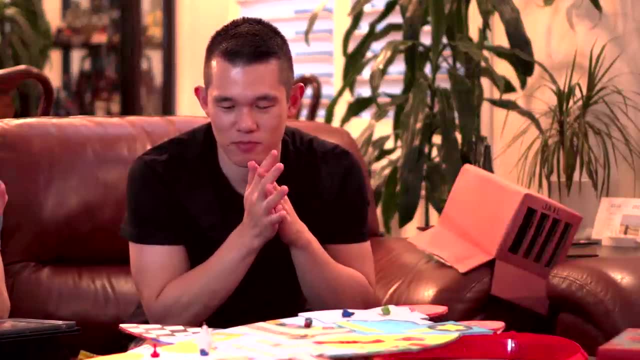 Which, if you notice, that's what she paid with, which is there's no distinguish between Looking for your, for critiques now, Things that you think were similar, things that you think were not, you know, and pros and cons, that kind of stuff. 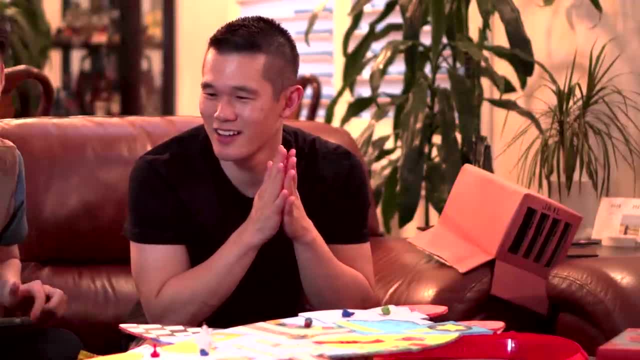 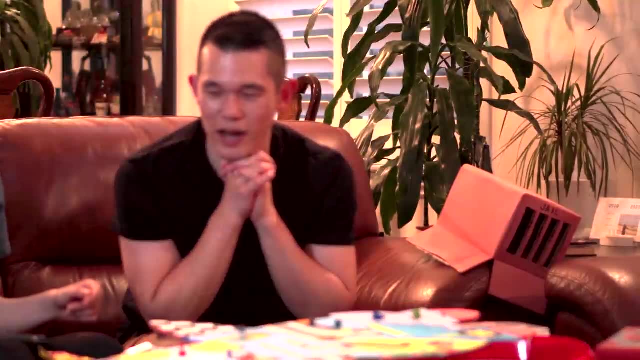 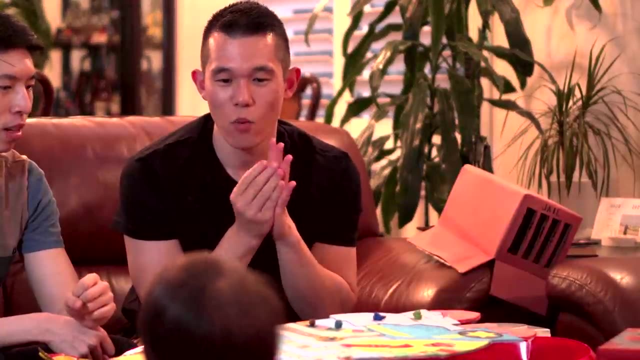 Are you allowed to rewrite the rules as you play? So yes, Oh, really, There's extra cards here. The blanks, Ah, little pencil, It's so accurate, But because of that it's also so chaotic In terms of pure wow factor when you like reveal it. 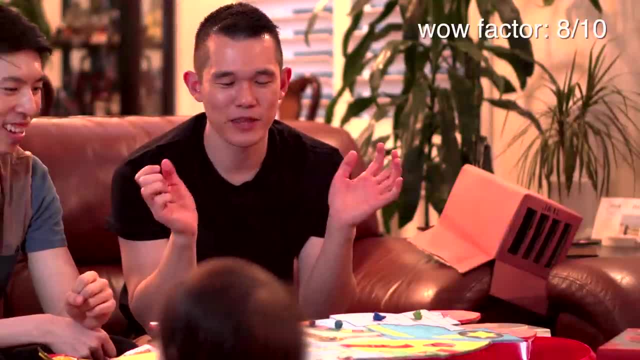 I was like: oh my God, it was like an eight. I was like, oh my God. But then a little bit confusion. it was like: oh, what's going on? There's so much going on, Like: how do you play this? 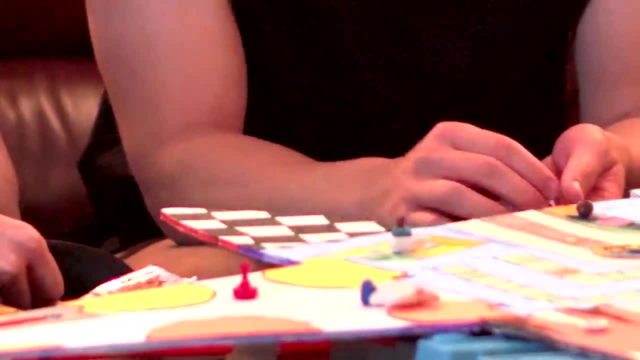 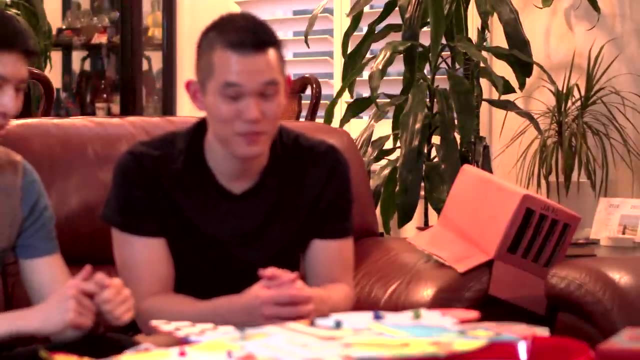 Is that checkers or is that like a? It's very accurate to the specifications. It's a nice case. That's a good, that's a really good way to put it. It looks like he bought several. he had several games. 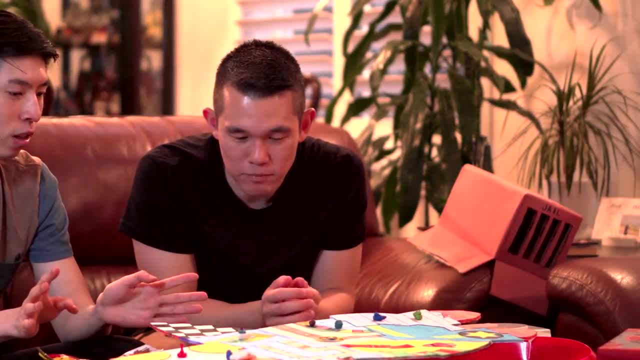 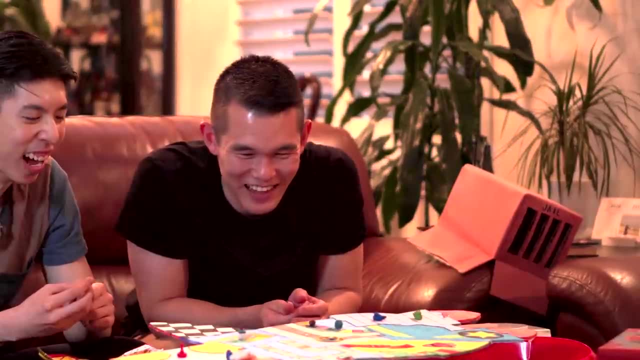 He just ripped it up and stuck it on it. So eight out of 10 for the wow factor or overall. What are there? Like accuracy- I think accuracy is probably higher Like a nine, Nine. A 10 would be a remote controlled car. 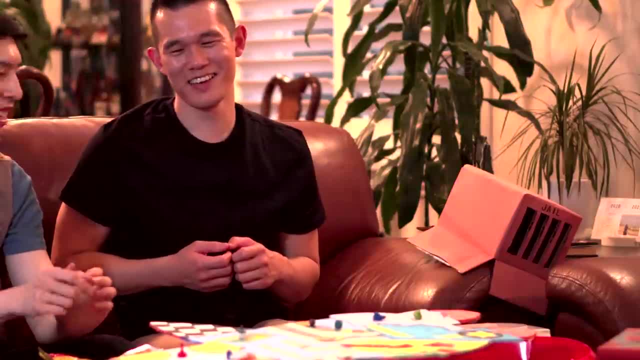 Yes, That's a good one, And then With a little button, you can sit on it. I don't think you'd ever sit on it. I didn't even sit on it, I know. Oh, we didn't like do this. 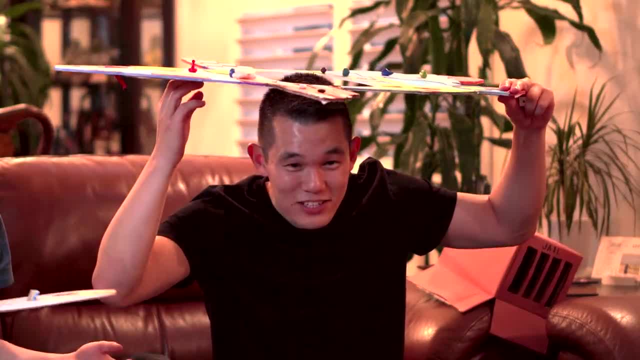 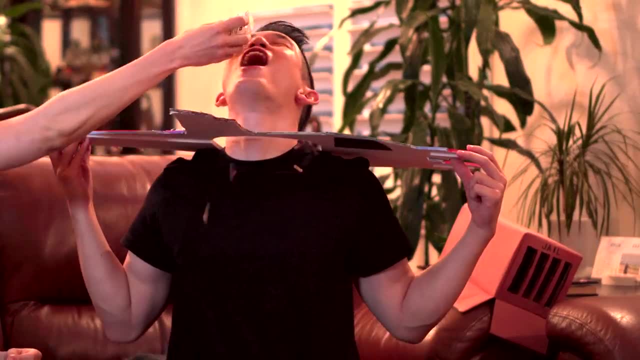 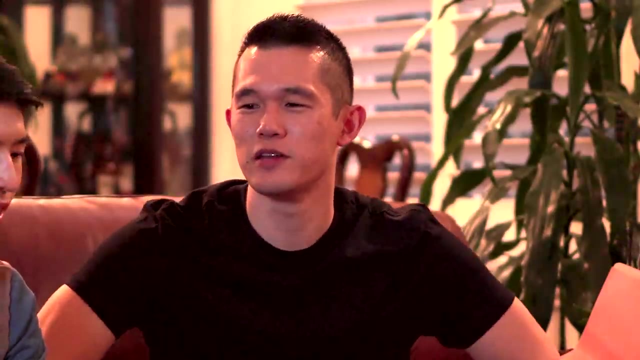 This is Starving Starving Sea Star Time. Starving Starving Sea Star Time. What do you want to do? I wish I knew about the episode. Personally, I feel disappointed that, but I think overall I give it an 8.5.. 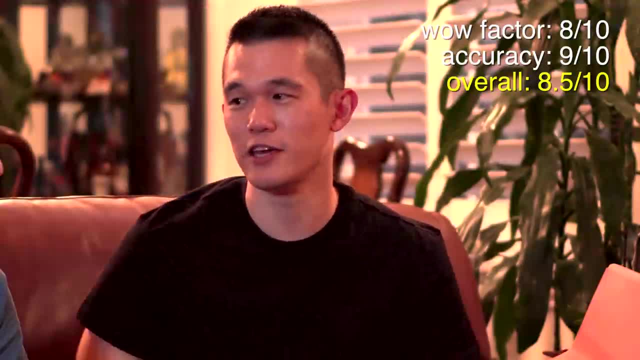 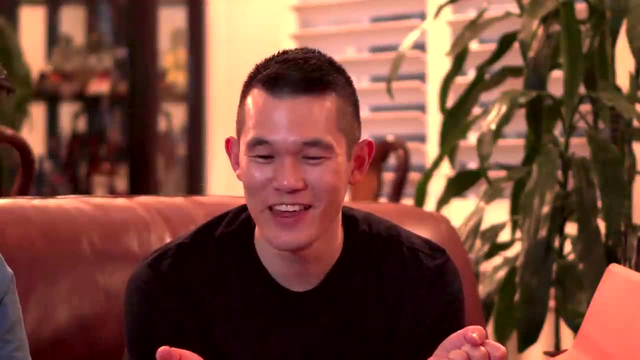 I wonder if other general like SpongeBob fans our age would know this game, or they would have to watch that episode too. Why don't we just play Okay, Roll the dice and then just figure it out as we go? Oh, I want the Patrick piece. 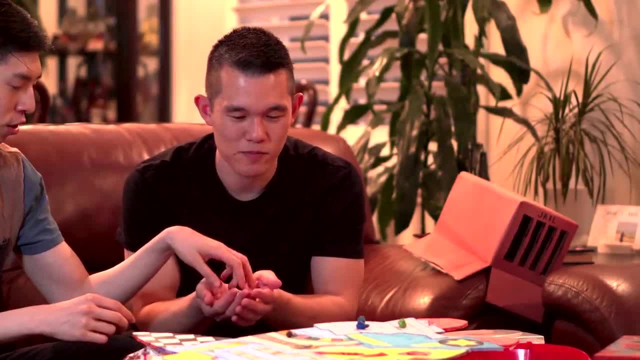 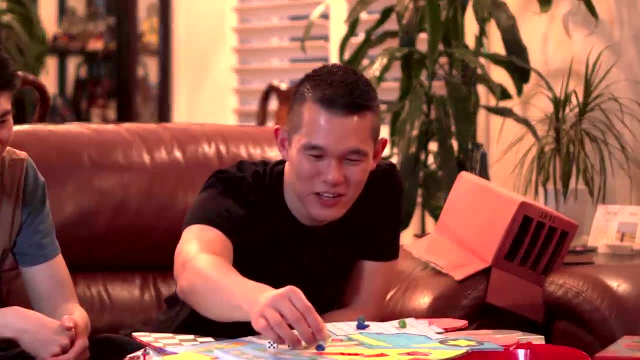 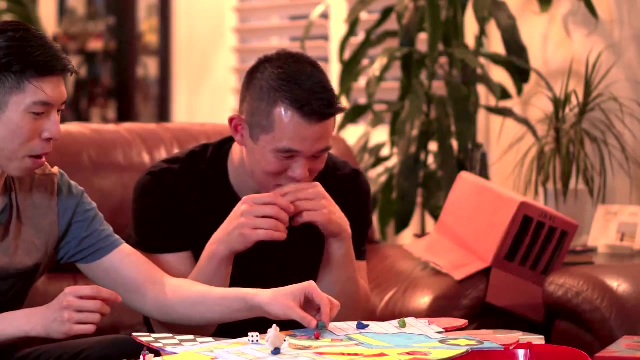 Okay, I'm going to be the acorn. Patrick goes first in the game. Six and six, 10,, 11, 12.. Oh, snacks, All right, my turn Beach for a property. Nine Travis Tyson. 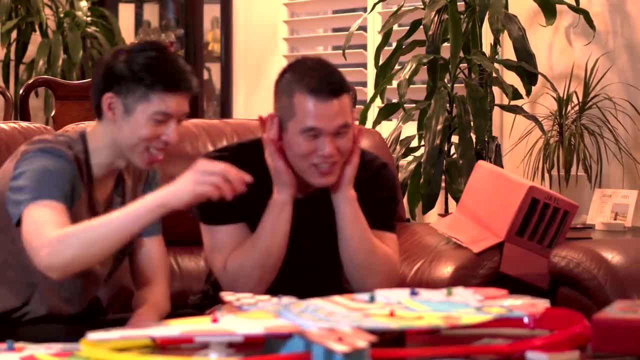 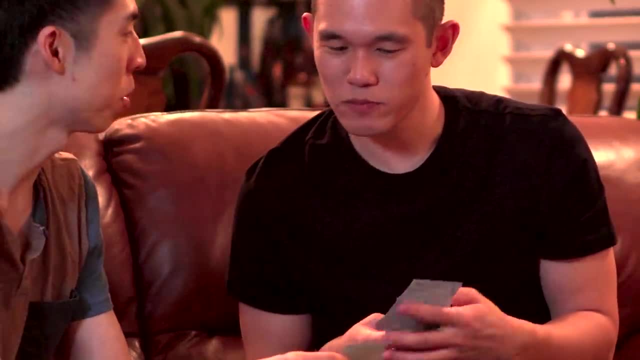 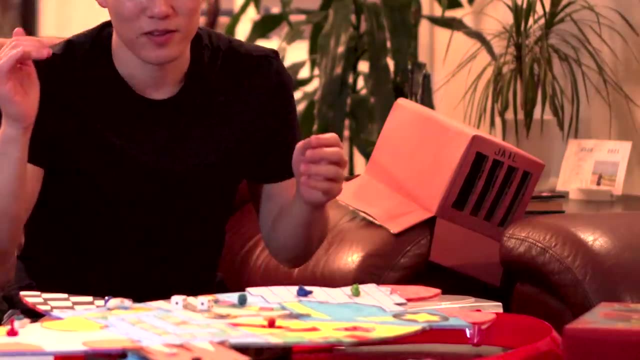 10,, 13,, 14.. Five, six, five, four, three, two, one Game over. Do a surgery? Have to pick a surgery card? No, I have to pick it, It's all you do. 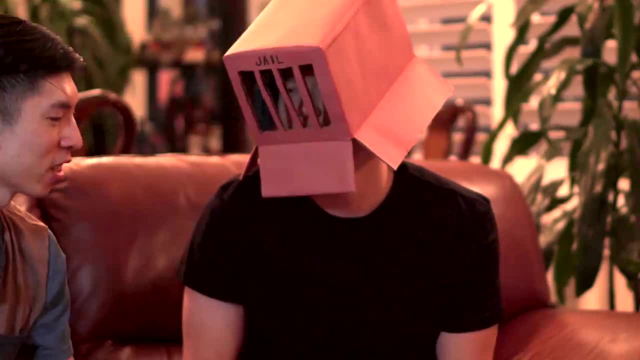 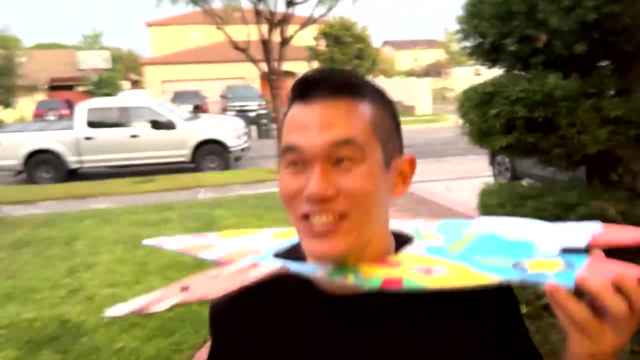 Is it? Yeah, Remove heart from any player. Oh See, Oh, But I don't have a heart. I'm an octopus. There's a hair on it. Yeah, It's like a reindeer Six. They only brought one dice. 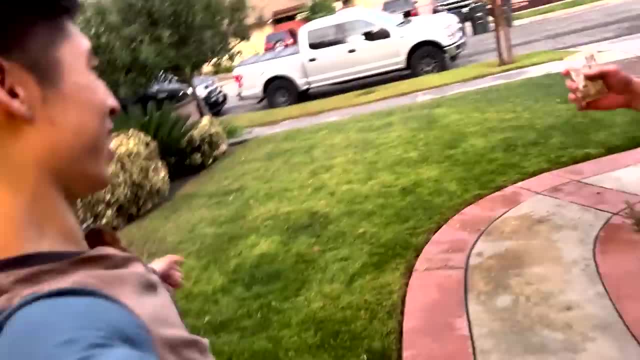 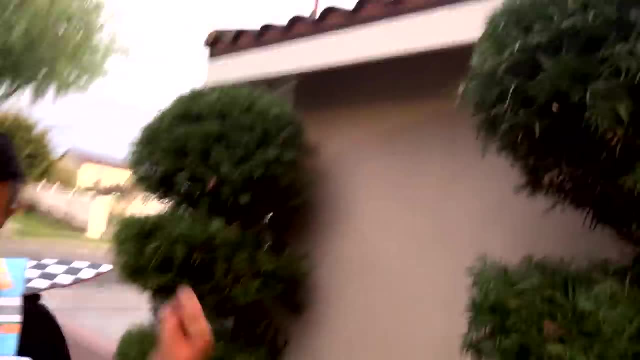 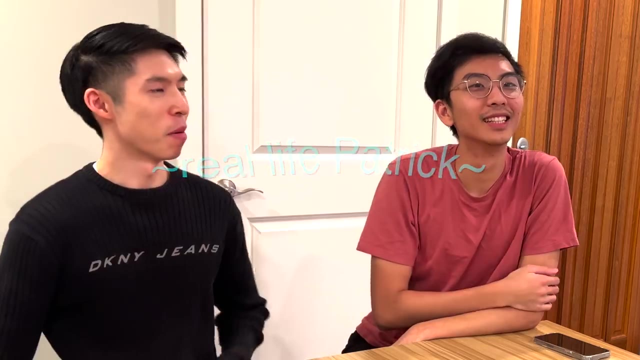 Six do a dance. One Oh One, We all win. After my fun playthrough with Sean, it was time to reveal the game to my friend Patrick, but not without a little prank first. I'm here with my friend Patrick and we're about to. 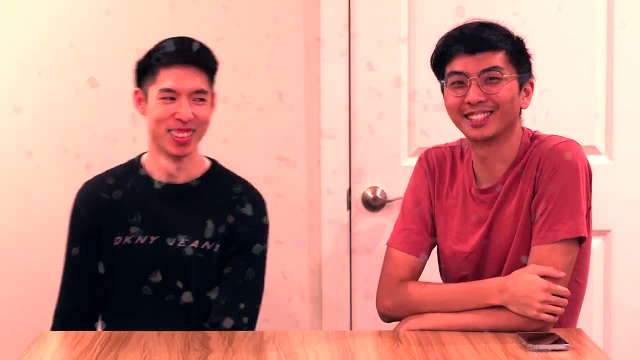 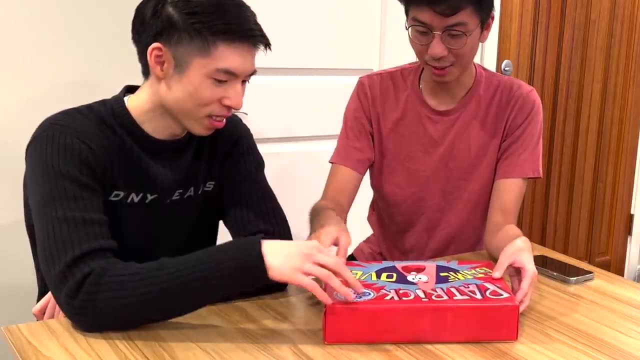 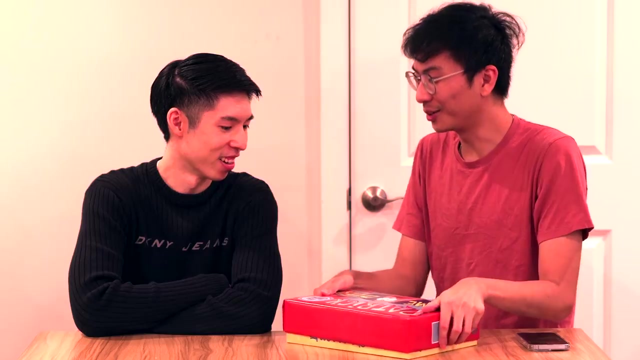 reveal to him. Patrick, the Game Hi Ready. Yeah, Oh, wow, So you made this as well. Yeah, I got this printed on um wrapping paper and then I wrapped it. Oh, You printed it on wrapping paper. Oh, I already. 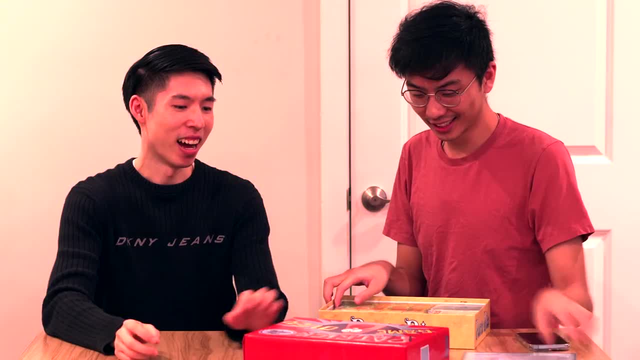 saw that, Oh, It's a trick. I didn't actually make the game at all. This is just a prank Prank. I'm just kidding. I actually did make the game. I had to go get it in my car. 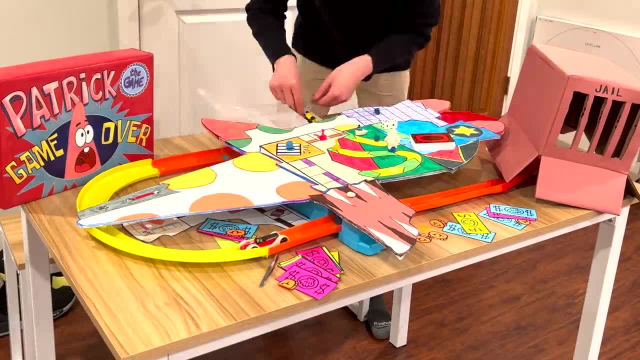 Oh. So I went to get the game in my car, set it up and gave Patrick a blindfold for the reveal: Oh, there's a table. Oh, don't don't wanna look. Oh, Oh, Oh, Oh Oh. 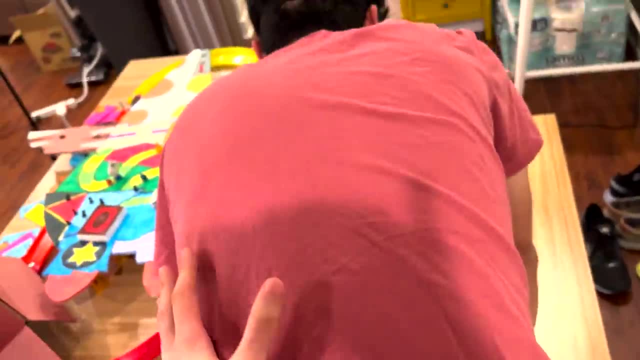 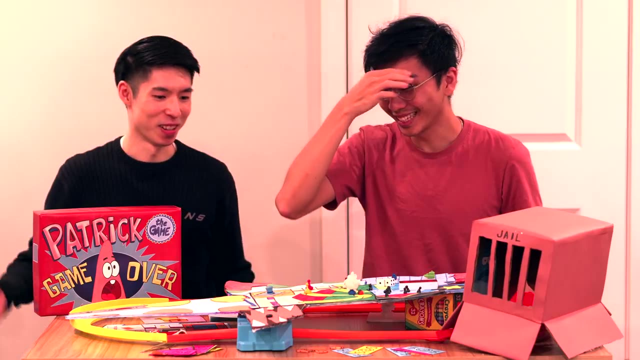 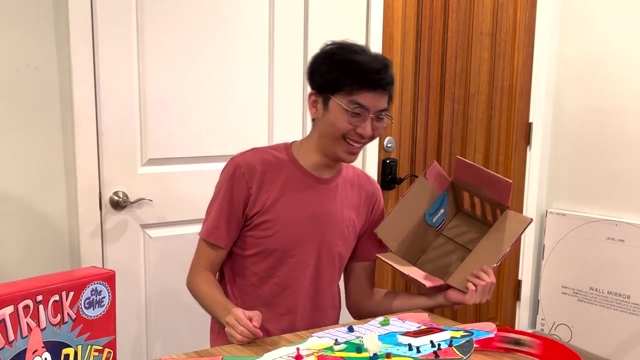 And then you're a hand to the left. Oh my god, There's a chair. Okay, yeah, Have a seat. Okay, Are you ready to see the game? Oh my god, We had to do this. What the hell. 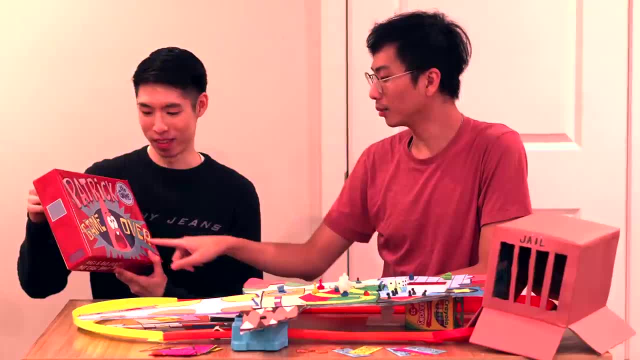 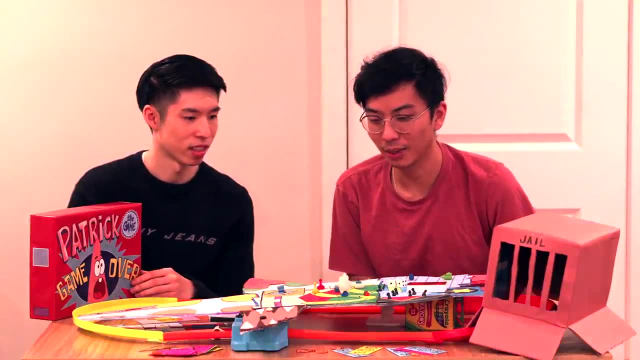 Do you remember this part? This was at the end. Yeah, I had it redrawn. Yeah, I had this redrawn. See it's high resolution. Yeah, Oh, my goodness. Okay, so you actually made all this. Did you draw this though? 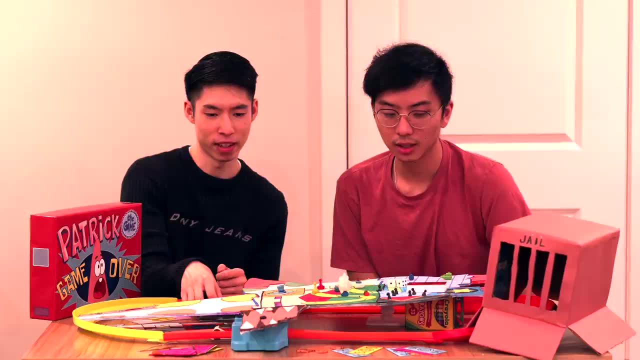 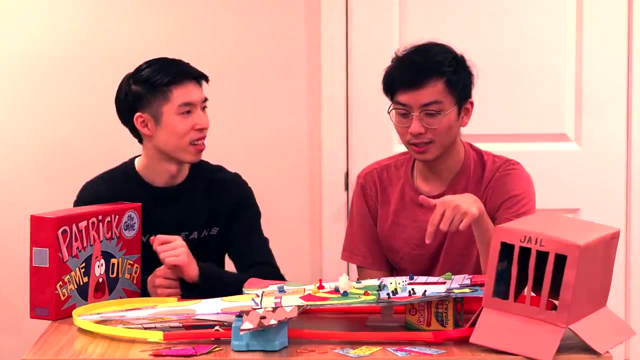 Yeah, I drew this. You made this. You drew this yourself. Yeah, I drew it myself. I cut it out and everything. What's missing? part of the floor, What's missing, Like the places that Sandy was going on. That's why we have extra. 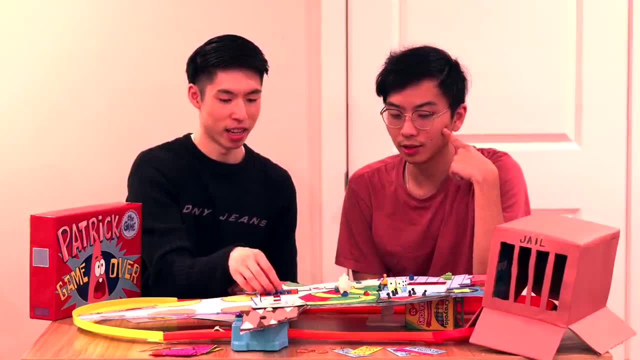 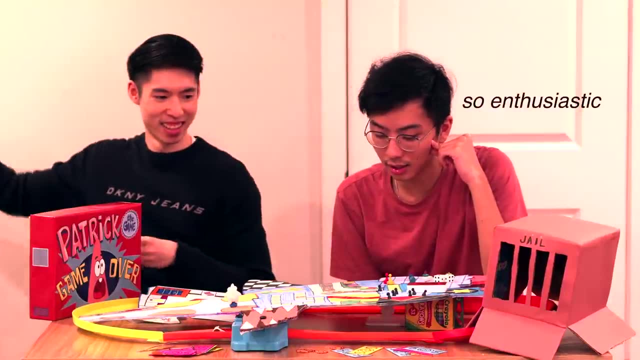 layer here. Oh What? Oh, so there's more still. You're not showing me yet. Uh-huh, Uh-oh. Oh, here it is. This is where Sandy was. This is where Sandy was. Okay, now you still. 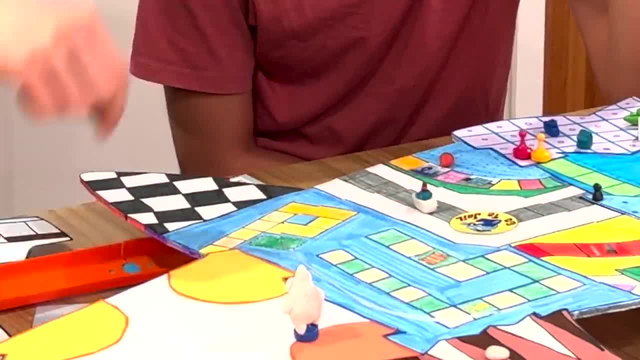 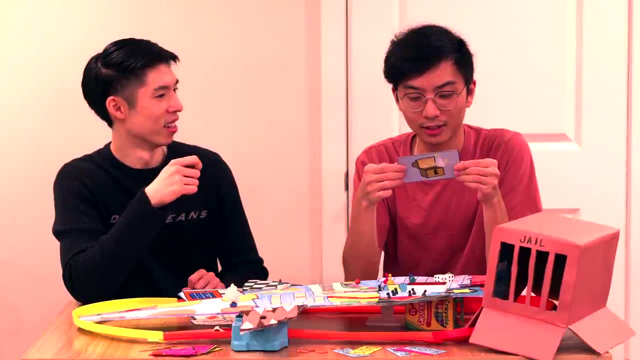 need to show me where SpongeBob was. He was here and he landed on Treasure. Oh yeah, So then, when he got the Treasure card, it was his driver's license. Yeah, You made this too. Uh-huh, Wow, You took this off. 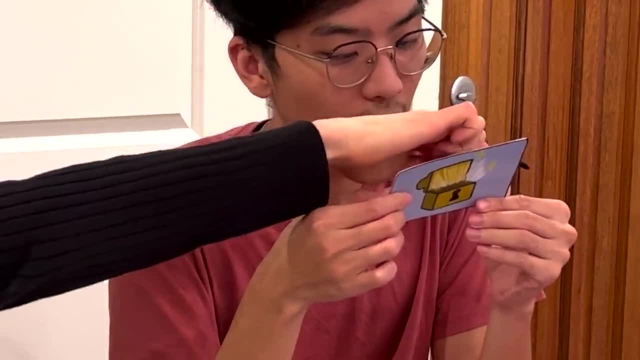 a screenshot too. This is a screenshot, except I did some Photoshop right here, Oh, Um, because his thumb was covering it, His thumb, Yeah, Oh, when he was holding it He was like driver's license, Driver's license. 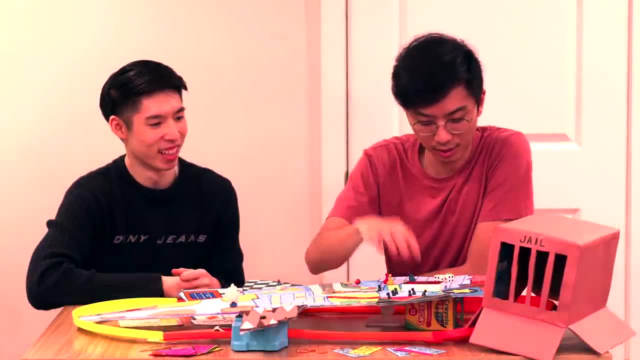 You don't have the remote, the controller. Oh, you're right, I don't have that. I don't even remember seeing this thing. This is just in some of the shots. Well, the surgery, Where's the bone place? Oh, 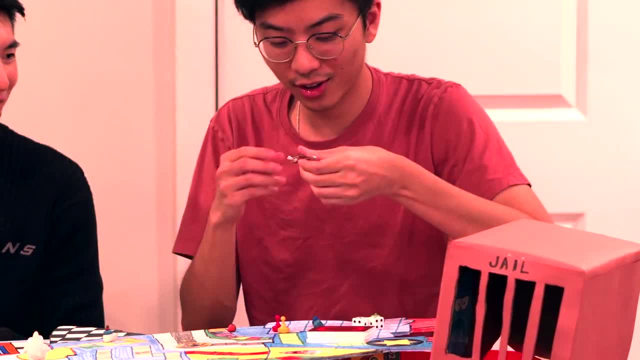 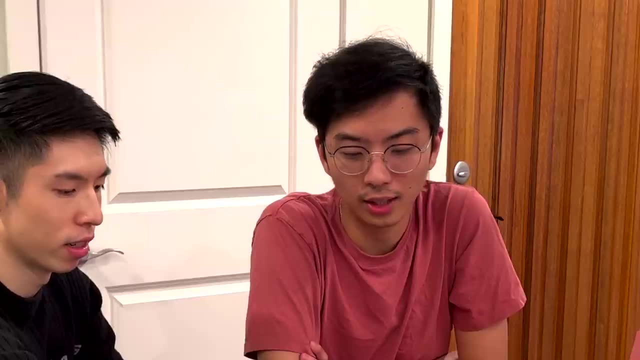 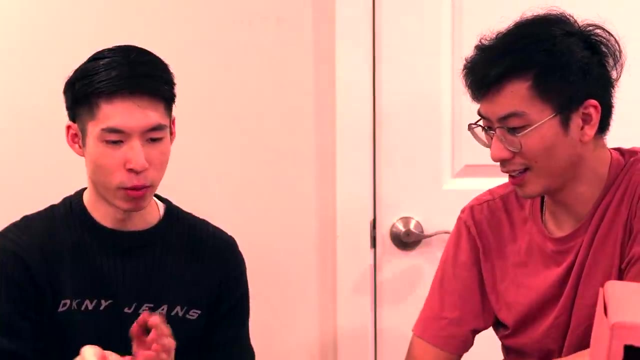 Okay, there, Okay, Oh, Nice, I got a bone. How long has this project been? One or two weeks of working on this, And then I've been editing for like two weeks. You want to do just like a random playthrough? Yeah, See what happens. 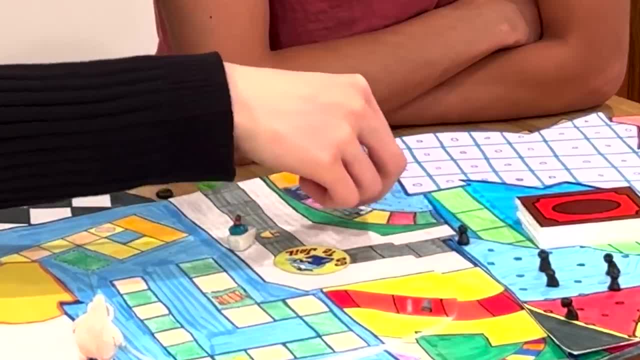 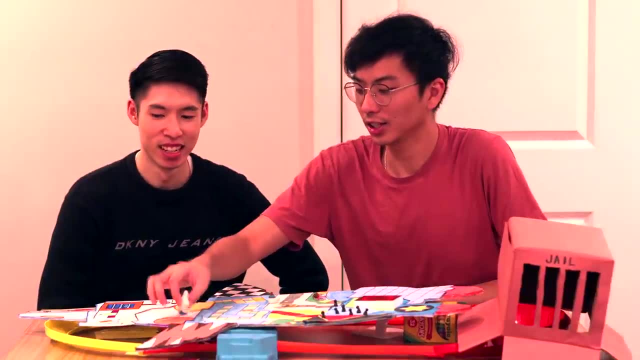 I'm gonna go first. Okay you go. One, two, three, four, five. Wah, wah, wah wah, Lose a turn. Okay Nine, I'll start here: One, two, three, four, five. 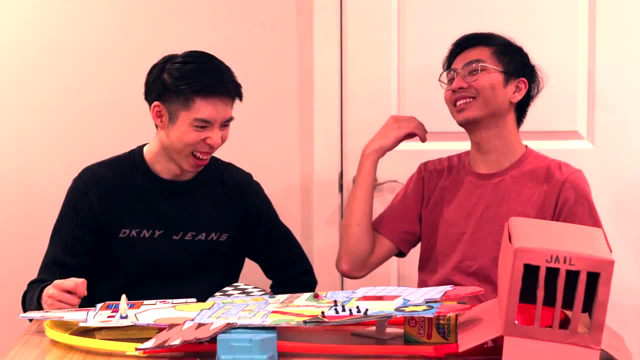 six, seven, eight, nine, eleven, ten. There's no other space to go back and forth. I lost a turn. It's your turn. Oh yeah, that's right, It's my turn. Four, I'm like one. two. 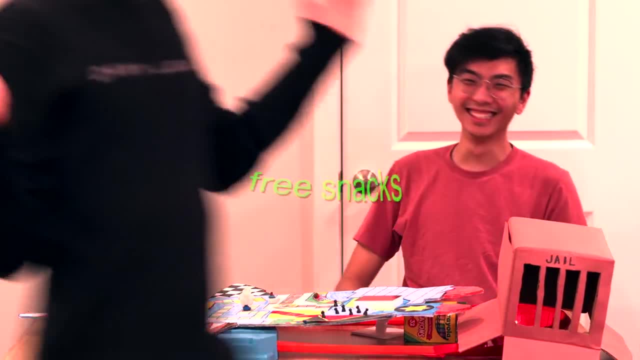 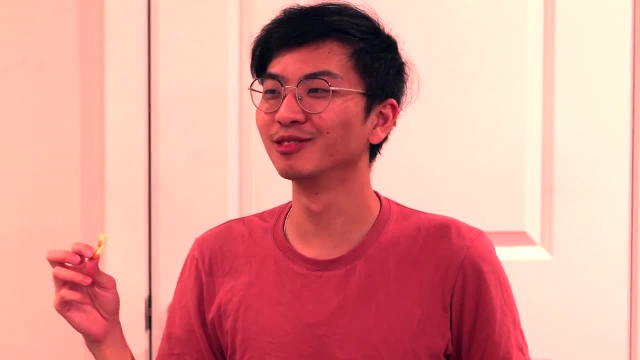 three, four, Woo. Free snacks, Free snacks. These are my favorite snacks, by the way, So good, Yum. Okay, is it my turn? Yeah, go Nine. One, two, three, four, five. 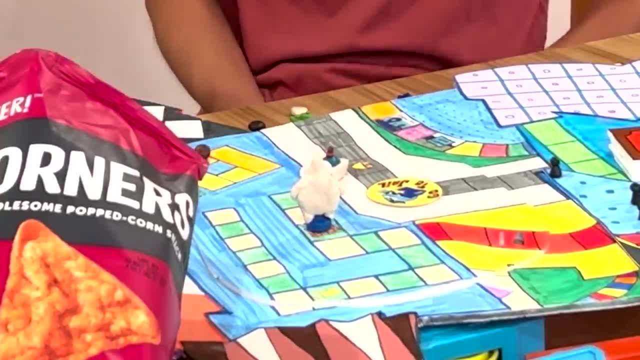 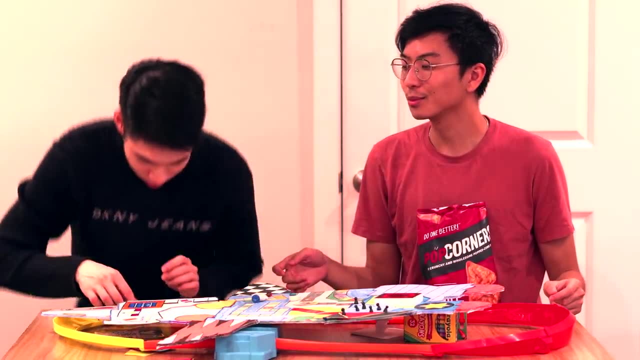 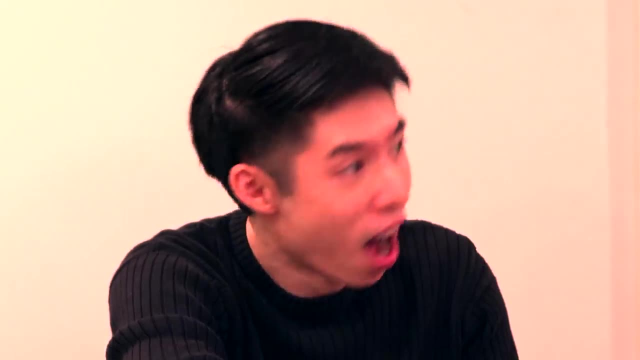 six, seven, eight, nine, Drive or slice Nine. Oh, you can go around nine times. Oh, You can go around nine times. Oh, you're right. One more time, Yeah, one more time. I want extra. 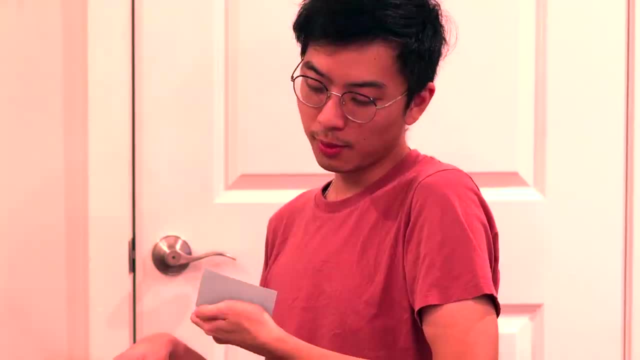 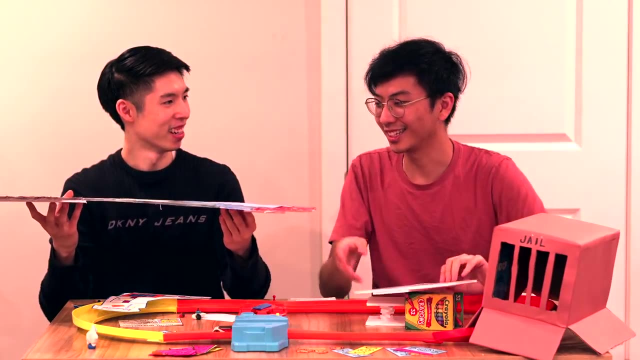 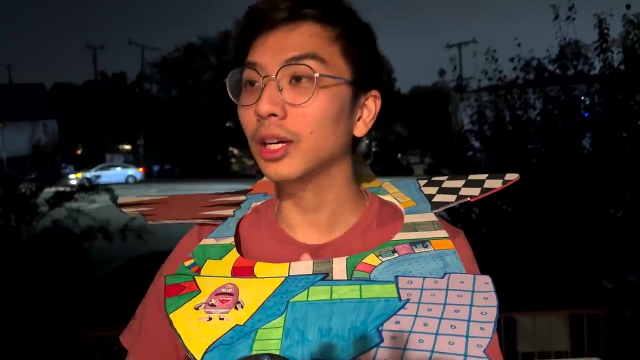 One, two, three, Woo, So free, Remove heart from any plate. Uh-oh, This comes off. Would you like to try it on? Yeah, give me Ooh Time to go outside. Three, Three is jump three times. 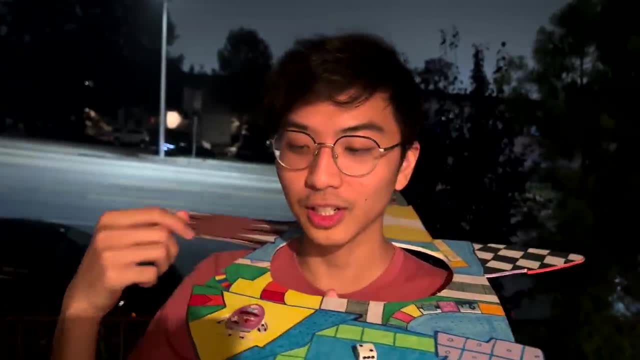 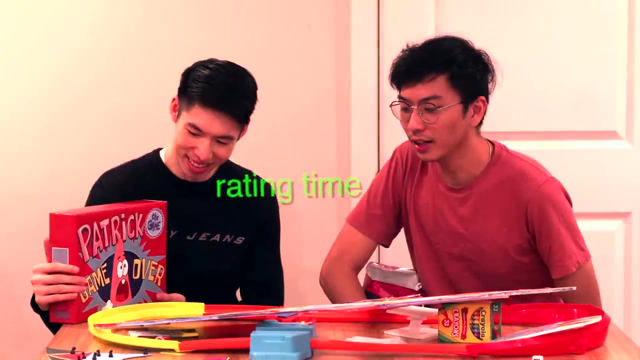 Jump three times: One, two, three, Two. If you roll a two, it's silly face. I got a one. I declare myself as the winner. Um, I think everything is like really close to the show, Like it's pretty spot on, I'd say like. 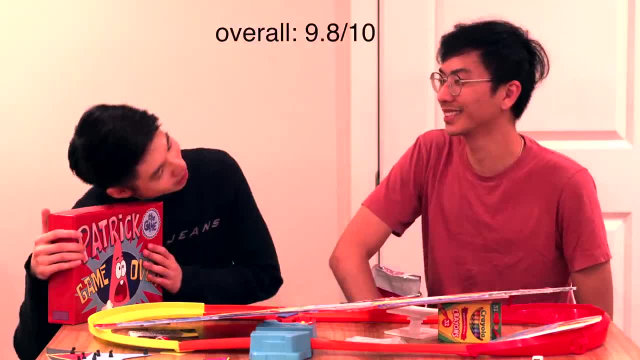 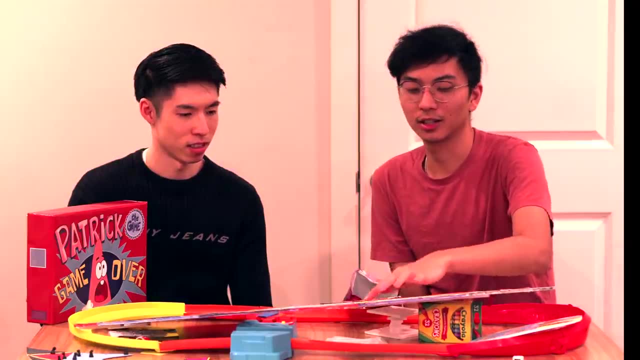 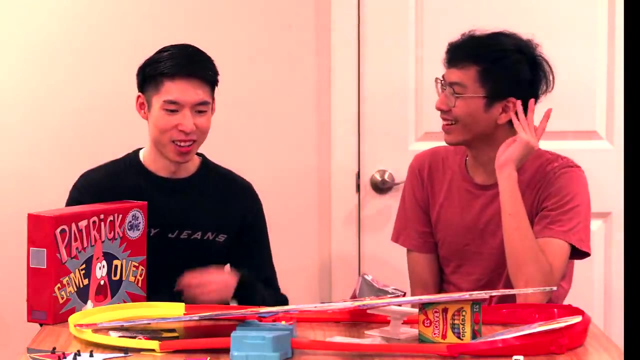 nine point eight out of ten. Oh, my gosh. Eight plus Nine point eight out of ten. The only parts where you lost points on is: you need a little work on the art finisher and then maybe if the snacks was coming from the middle. Oh, you're like shooting. 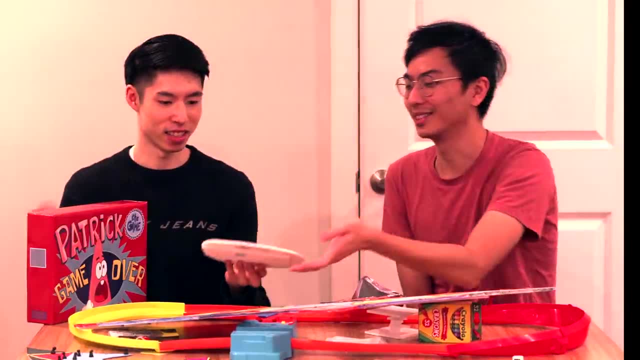 out of the thing. Yeah, like, obviously I don't expect you to like have something to shoot snacks. I was trying to, I was thinking about it. If I use like a baggie in here, and it had a rubber band I could have. 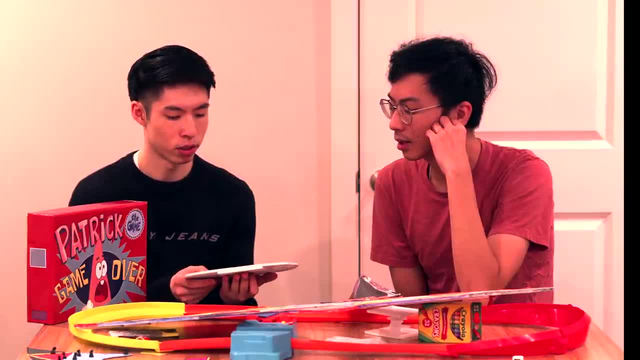 half a snack in here and pull the rubber band back and then shoot it out, But then I couldn't find pretzels. would be like super small. Yeah, You're missing the remote control from the track. Do you want to guess what this is? 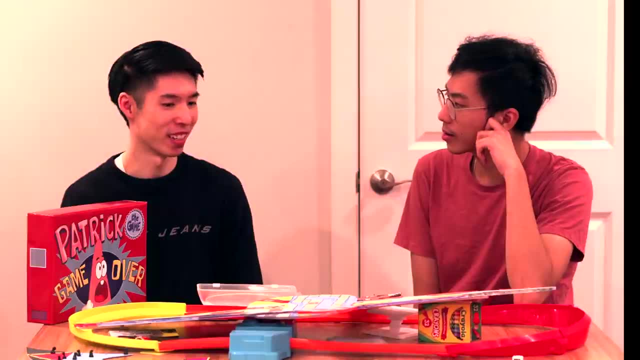 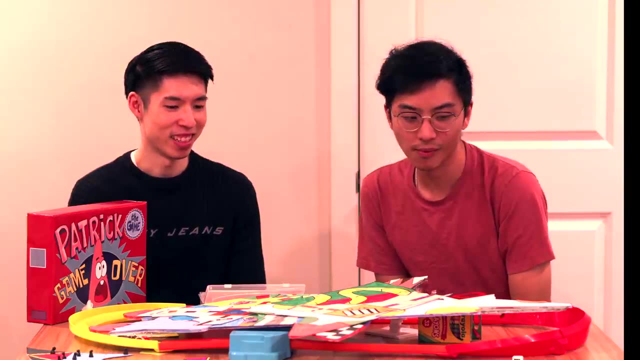 It's Twister. Oh, I didn't realize until later. Good work, though. Like I, I'm actually like surprised you made this life-sized. Aw, thank you. With a nine point eight from Patrick and an eight point five from Sean, I was pretty. 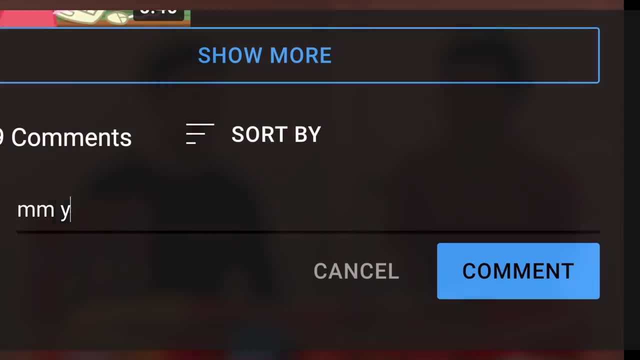 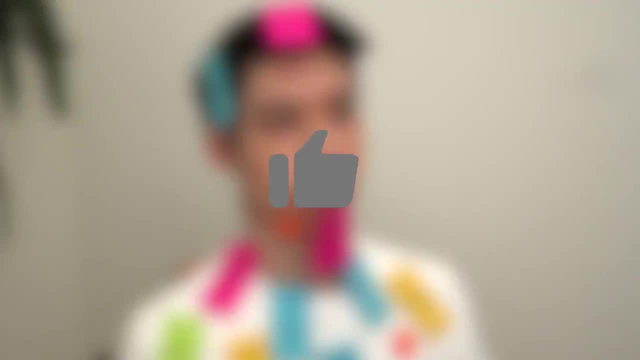 satisfied with my nine point one five average rating, But what do you think Anything I missed? Yes, I already know the remote control's missing. I spent months working on this project, so if you could please give me just a little, like I would.